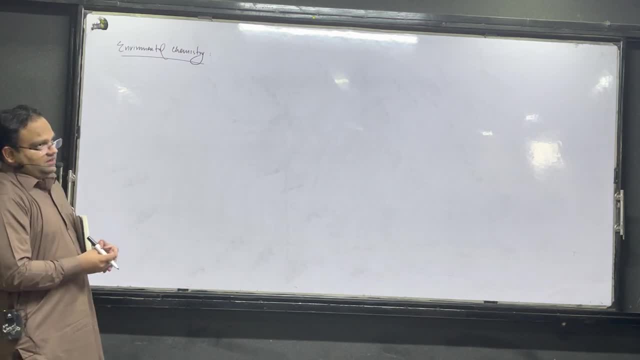 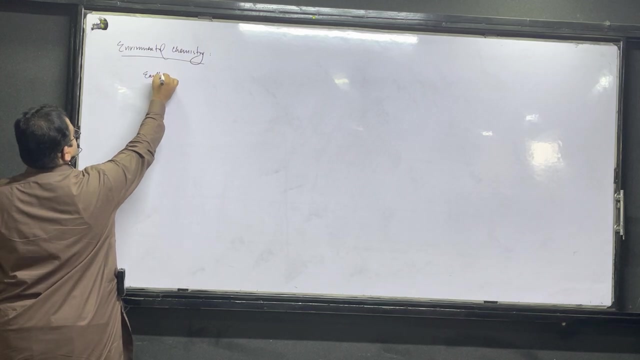 So, graduates, we will talk about this topic of environmental chemistry in this chapter. In different types of environmental chemistry, it is said that the whole world is divided into different zones. The whole earth is divided into different regions, The one which is called as lithosphere. and another one is called as biosphere, and another one is called as hydrosphere and another one is called as atmosphere. The whole world is made up of four regions of scientists: Lithosphere, biosphere, hydrosphere and atmosphere. Lithosphere is the region of the earth, The crust of the earth. You can say that it includes the earth crust In which we get minerals from the earth. We get minerals from the earth, So what is generally called this region, Lithosphere. 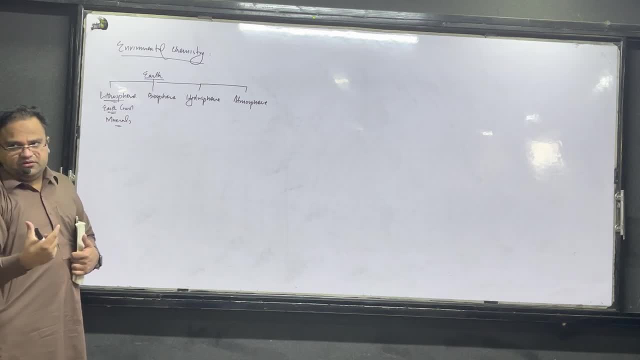 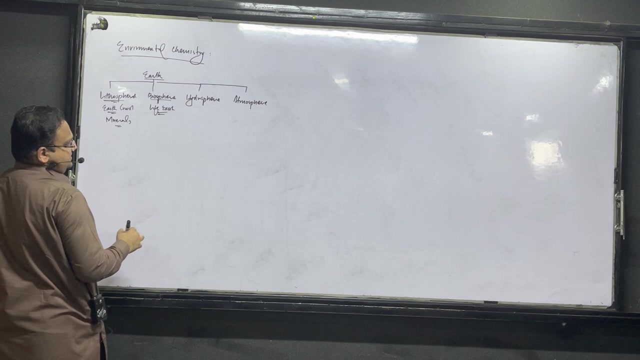 The earth crust corresponds to the mud area From where we can extract materials, minerals and mines. That is included in the lithosphere. The biosphere is known to be the region of the earth where life exists, Where living organisms exist, So that one is called as biosphere. 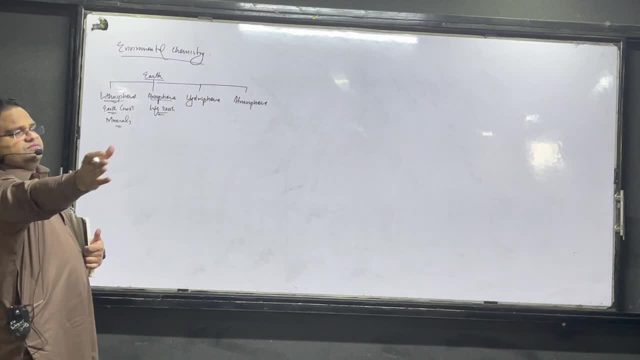 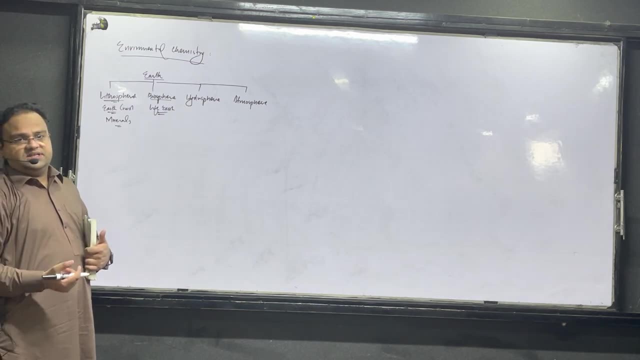 It is not like this. This portion is lithosphere and this portion is hydrosphere. They are fused in each other. It is like Karachi. You will see biospheres in Karachi, And what will you see in Karachi? Hydrospheres. 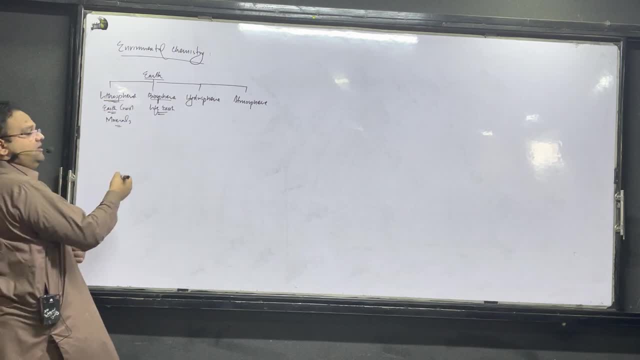 So there are mines in it. What will you see in it? There are fuses in it, But it is not like this. It is a full partition. Generally, we have this everywhere. Anyhow, the region where the earth crust is included is called lithosphere. 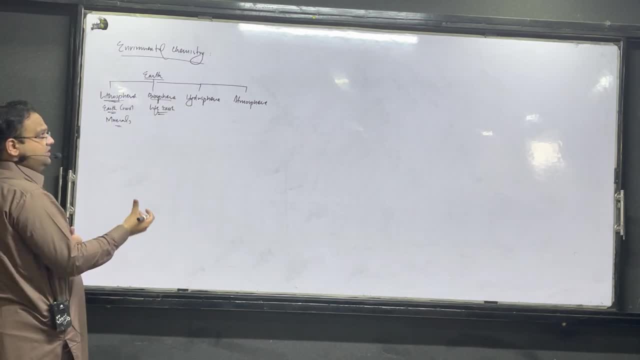 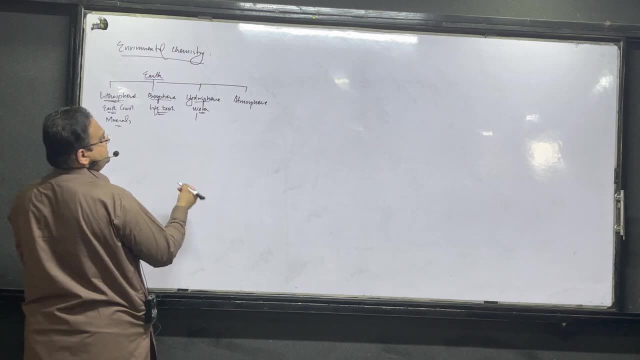 The region where life exists, For example, where living organisms live. It is called the biosphere- And that region which includes the water- The water that we have- is called the hydrosphere. We have the sea in it, We have the oceans in it. 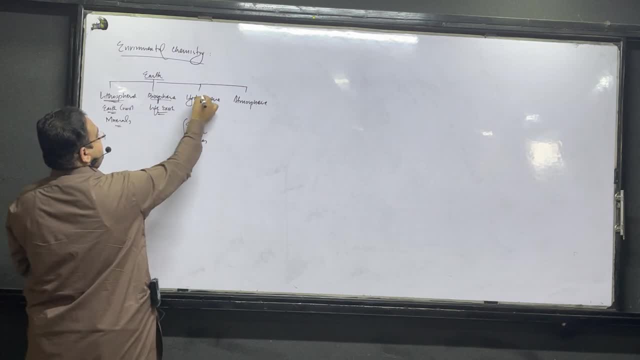 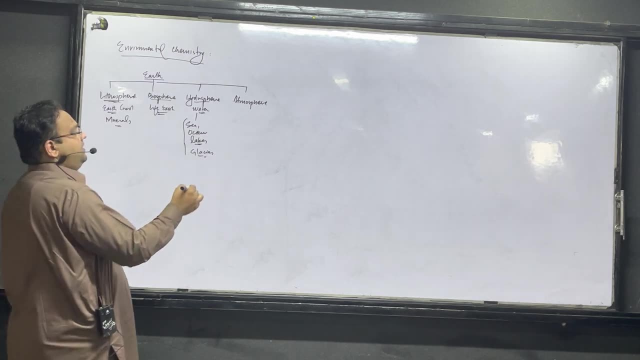 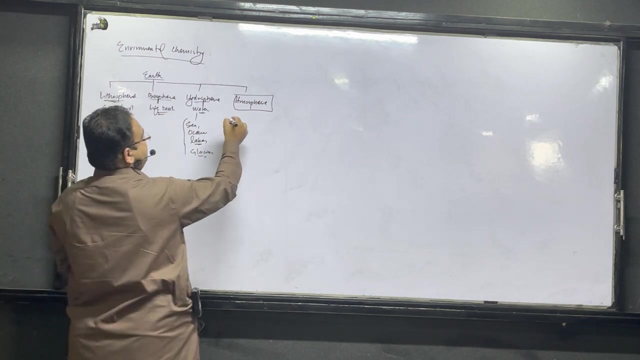 We have lakes in it. All these things are included in the biosphere, But even the glaciers are also included in the biosphere. And then we have a region which is called the atmosphere. I like its definition very much: Atmosphere. It is said that the blanket of air. 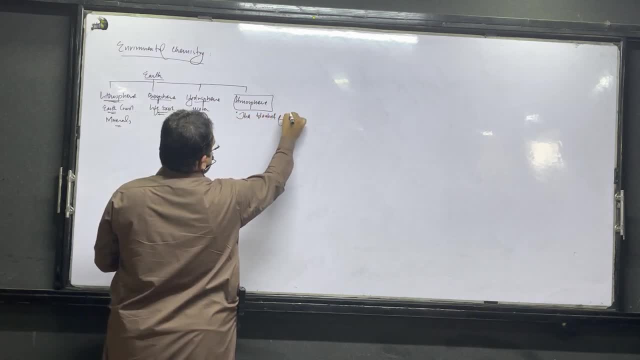 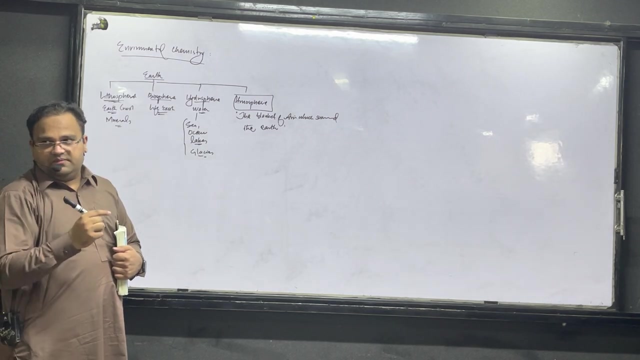 the blanket of air which surrounds the earth, which surrounds the earth, So that one is called as atmosphere, The region of the earth which is hidden in the air, So that region is actually called as the atmosphere In this environmental chemistry of yours. 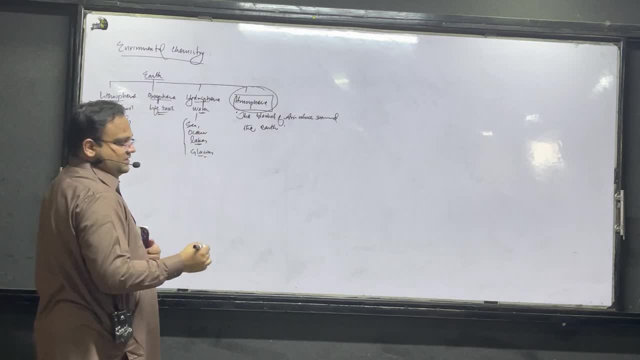 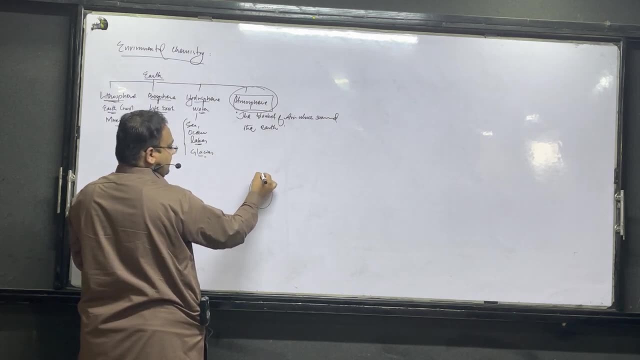 this mission has been broken. For example, what do you have to say about this Atmosphere? So, students, this is the earth, This is a beautiful earth, And in this earth we have a region, And this region is corresponding to the atmosphere. 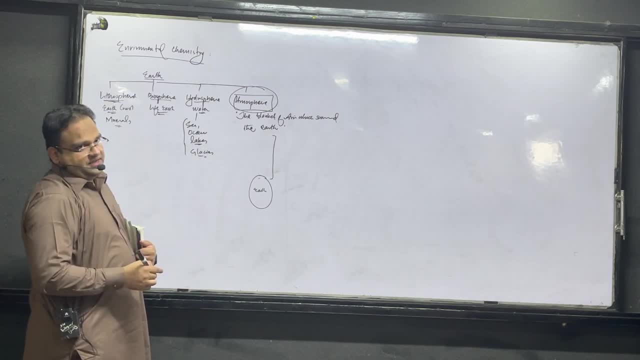 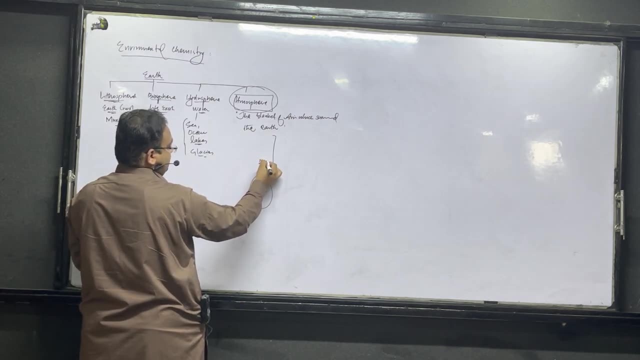 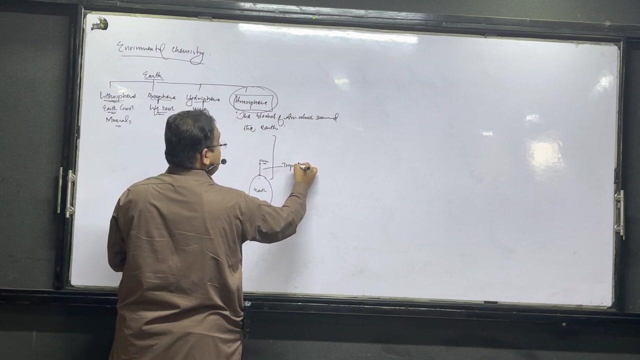 Now this atmosphere is classified into different portions: Students from the earth. if you go towards the ocean, from zero to one, it is approximately 11 kilometers, So this region is generally called as troposphere. What is called Troposphere? Then from 11 kilometers. if you go upwards, it is approximately 50 kilometers, So this region is called as stratosphere, And then, if you go above 50 kilometers, it is approximately 85 kilometers, So this region is generally called as mesosphere. And then from 85 kilometers, which is above India, it is approximately 500 kilometers. So this region is called as the atmosphere. All the other regions are called as ionosphere, But it is also called as thermosphere. So let me tell you. there are four regions of the atmosphere Which are your regions? Troposphere, stratosphere, mesosphere and ionosphere are thermospheres. If we go up from the earth to the troposphere, then the temperature, if we do, the output. then the temperature is from 15 to it will go down to minus 56 degree centigrade. In stratosphere, minus 56 degree centigrade will go down to minus 2 degree centigrade And in mesosphere, 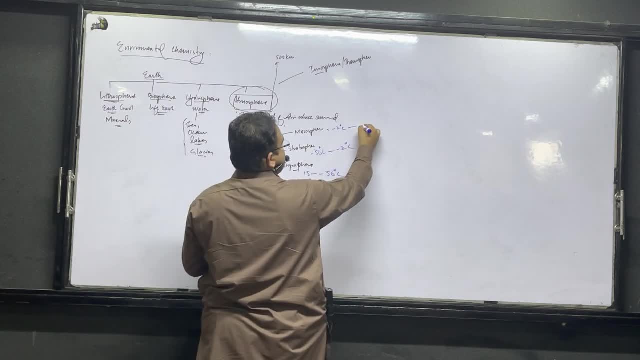 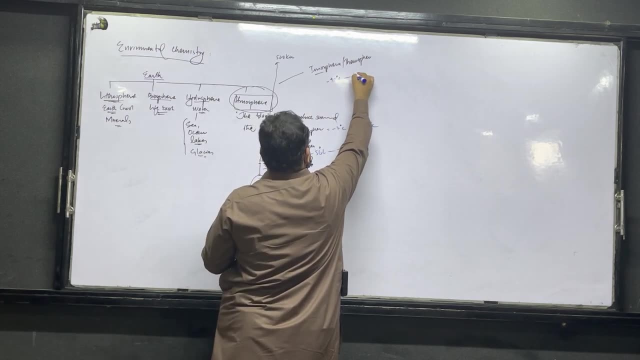 it is now over. so minus 2 degree centigrade we will have minus 92 degree centigrade And in ionosphere, if minus 92 degree centigrade is left, it will be 1200 degree centigrade. 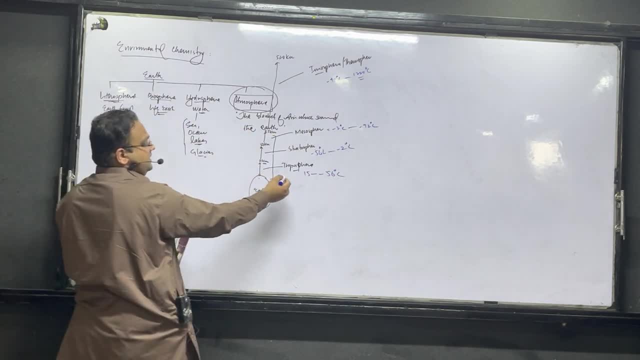 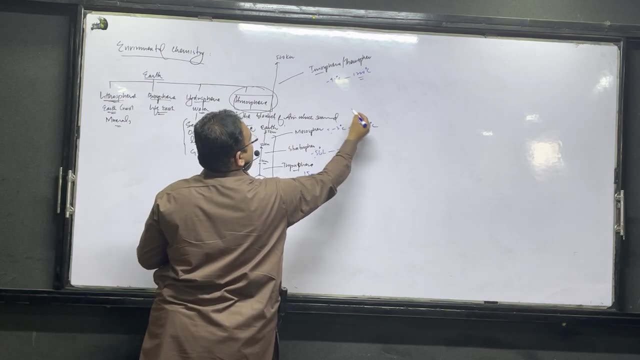 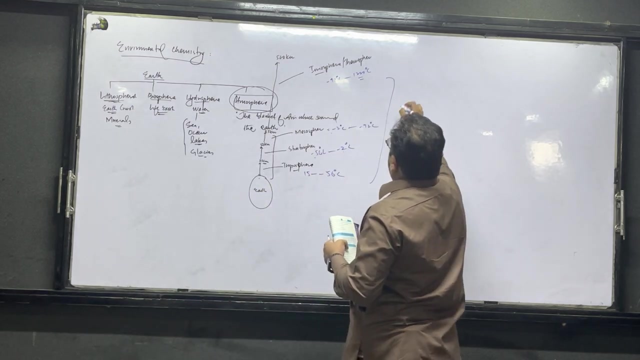 Now you tell me what happens to the difference between the two. Yes, Earlier temperature was lower, then the temperature increased, then again it was low and then again the temperature increased. The changes of this temperature. we call it inversion. What is it called in Sanskrit? 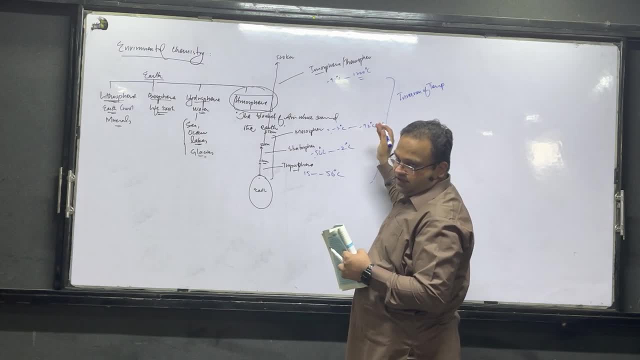 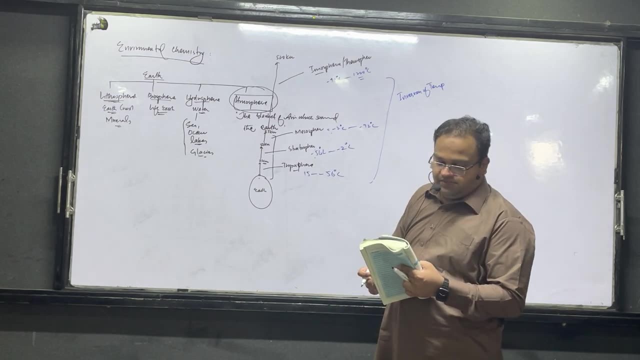 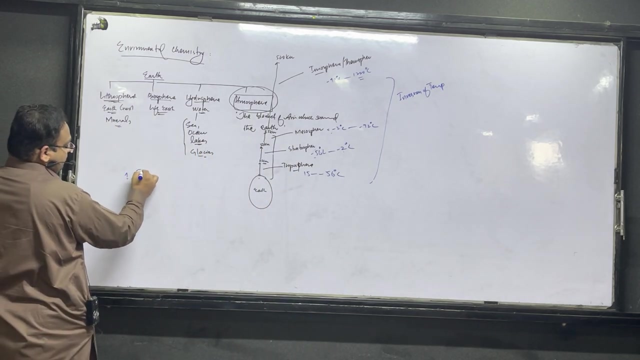 fond of. Sometimes it is low, sometimes it is high and sometime high. So they call it compression inver reserve. This is called the combination or the combination of the combination. In this, the first thing we need is the arrangement structure which we generally call the troposphere. Tell me what is the range of the troposphere: 0 to 11.. What is the temperature here? 15 to minus 56 degrees centigrade. Let me tell you something interesting. If you look at the height or distance of the atmosphere, 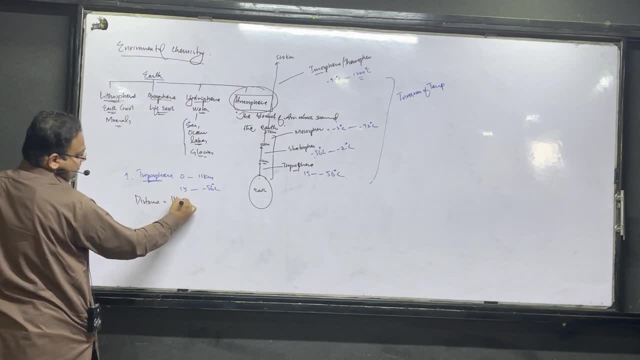 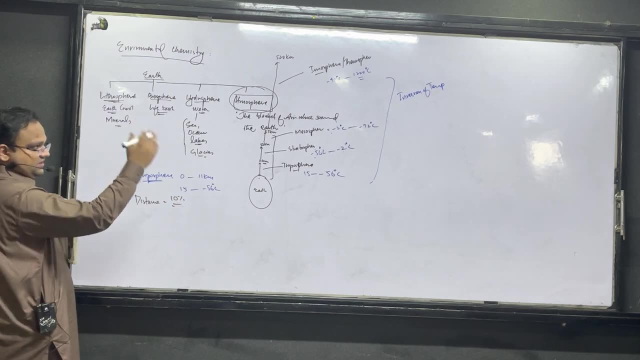 then, in terms of distance, the area of the atmosphere is 11 kilometers. Sorry, it is 11 kilometers, but it is 10% of the atmosphere. But in terms of distance, in terms of area, but if you look at it in terms of mass, 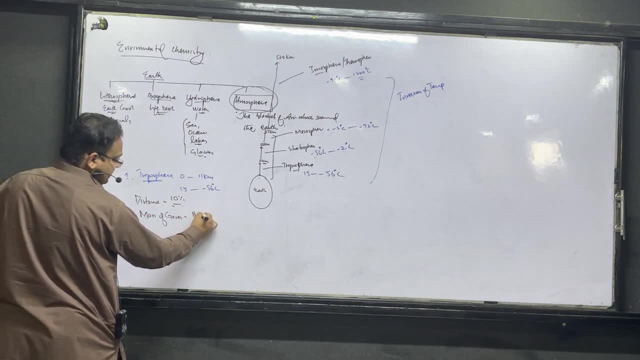 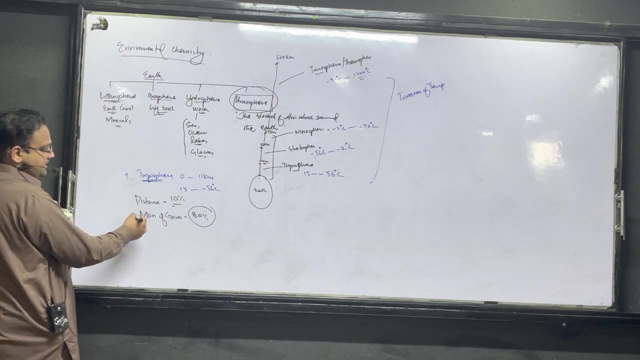 the mass of the gases, then the area of the atmosphere is about 80% of the earth. What do we have? Troposphere: This means that you have different gases in this troposphere. Now, what gases are there in this troposphere? 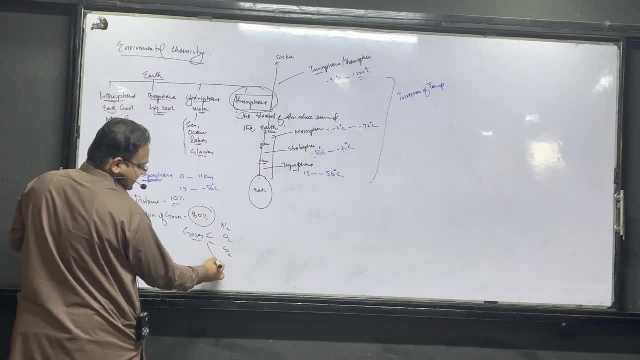 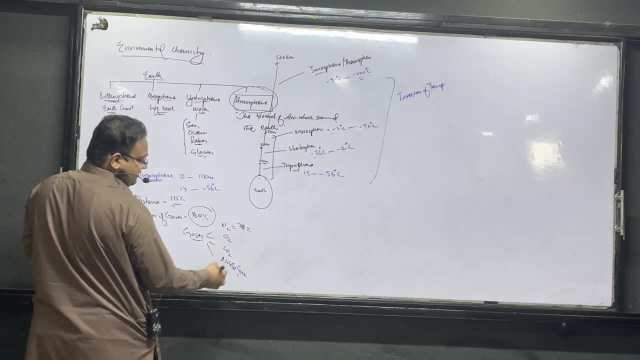 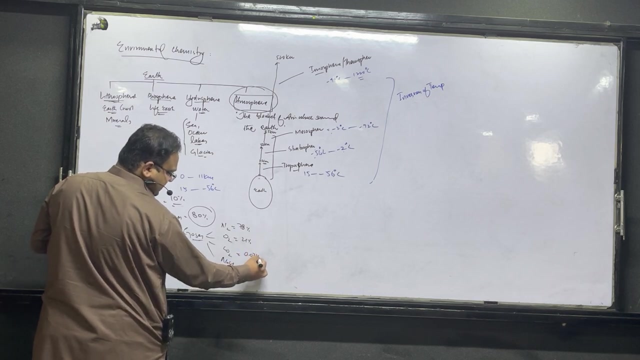 There is nitrogen, oxygen, carbon dioxide. and then what gases do? we have No gas. Do you know how much nitrogen is there? 78%, And oxygen 21%, And carbon dioxide 21% And carbon dioxide 2.03%. 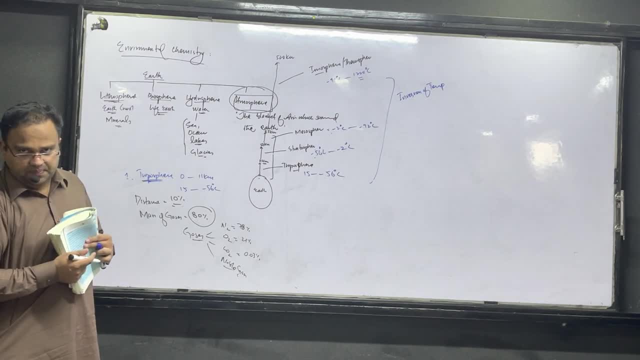 And this is the amount of gas that is present in this gas. So if we look at the quantity of these gases, in which region they exist, then what will be the answer? Troposphere. They exist in the troposphere, Now in the troposphere. 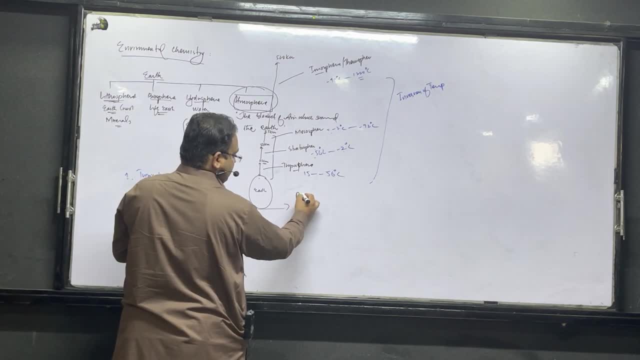 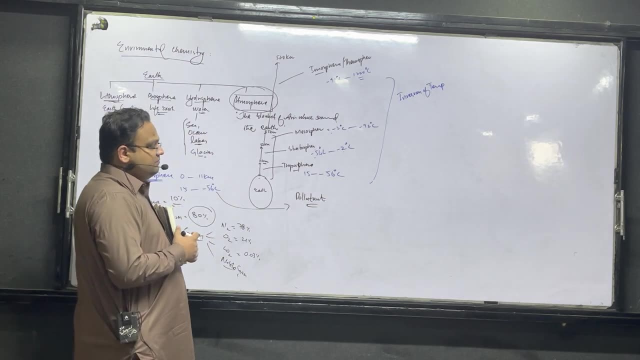 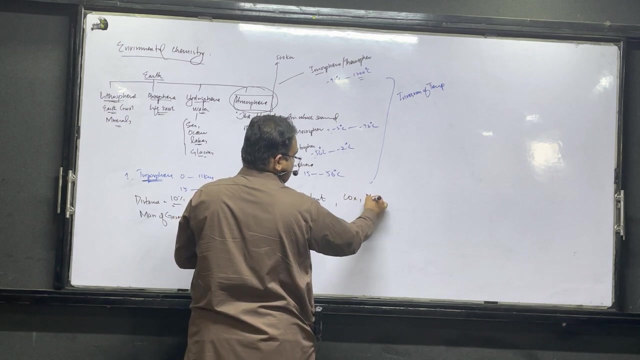 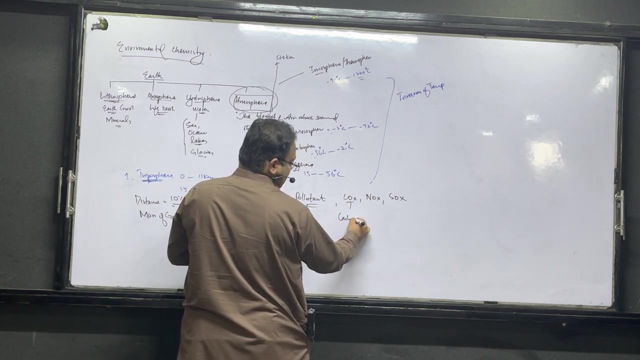 we have some pollutants, Pollutants Which pollute this environment. In the troposphere which pollutants are present? So in the troposphere we have cox, there are nox and there are sox. Cox is called carbon oxide. Nox is called nitrogen oxide And sox is called sulfur oxide. So in this troposphere we have monoxide and carbon dioxide And nitrogen monoxide, or nitrogen dioxide and sulfur dioxide and sulfur dioxide. These are called air pollutants. Everyone knows what air pollutants are. 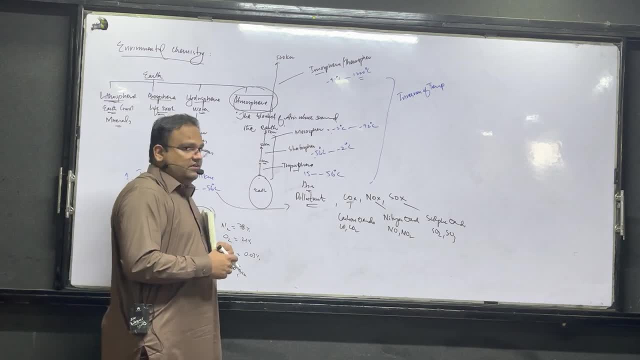 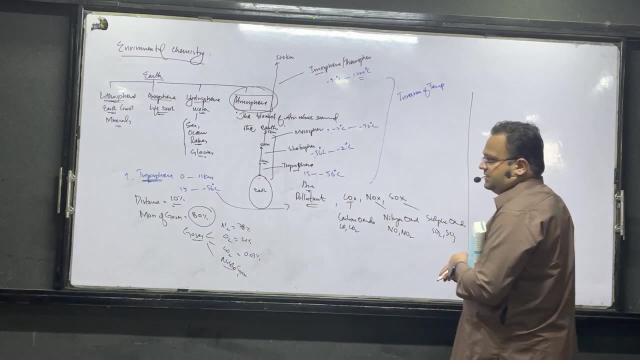 Yes, Do you know what air pollutants are? Yes, sir. Okay, Now we can discuss the different types of pollutants. Now, in these problems of air pollutants, we have one problem, And that is called as smoke. What is it? 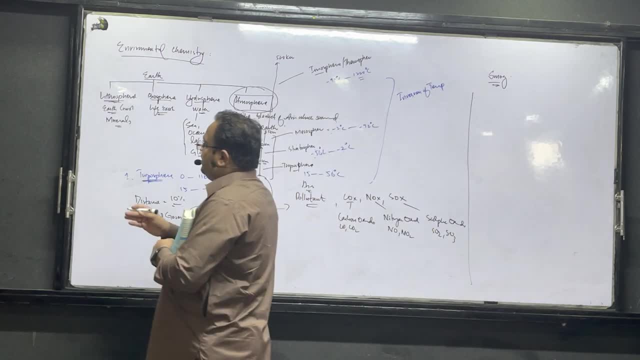 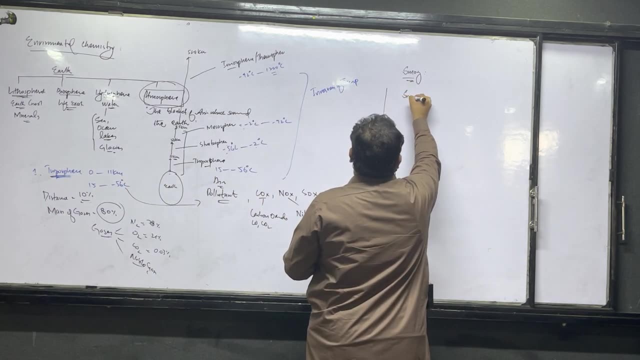 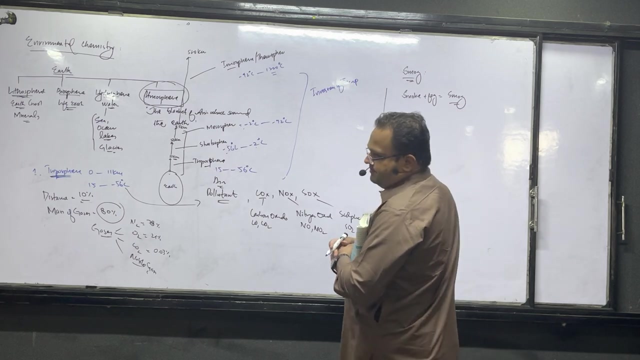 Smoke. Yes, smoke is also consumed. What is smoke? Two things come together. What do they come together? When smoke and sulfur come together, then what is generally consumed? Where does the smoke go? Have you read the chemistry? What is smoke? 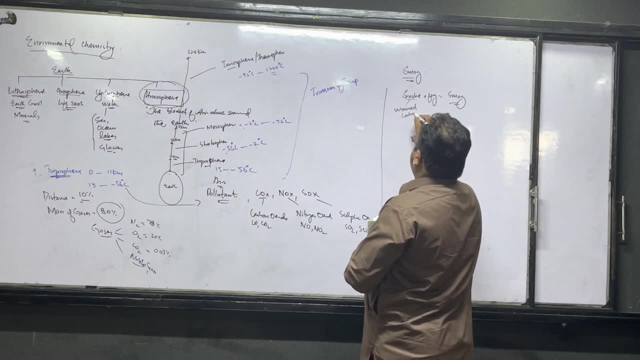 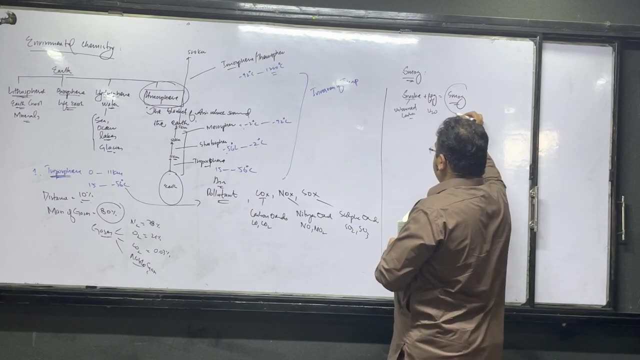 What is smoke? Unburned carbon? Do you know What is smoke? What is smoke And basically, what is smoke Water? This is what makes us happy. We make smoke. So how does the smoke make different things? 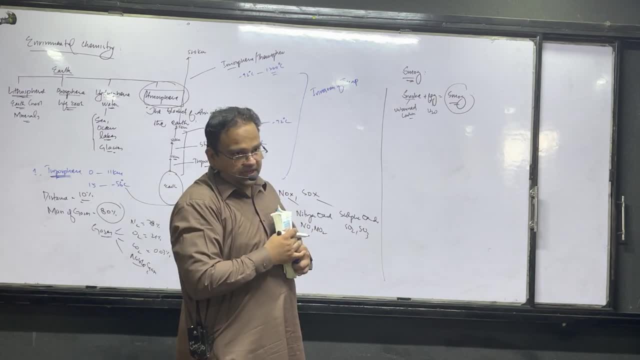 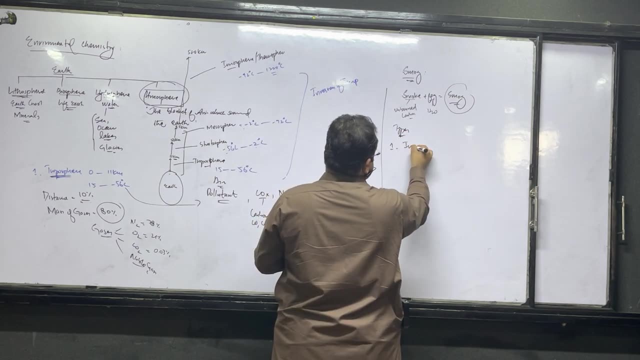 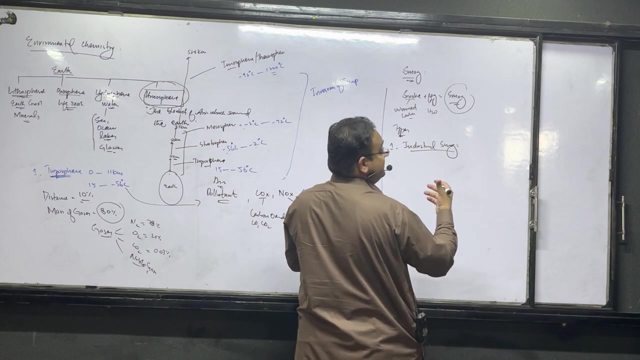 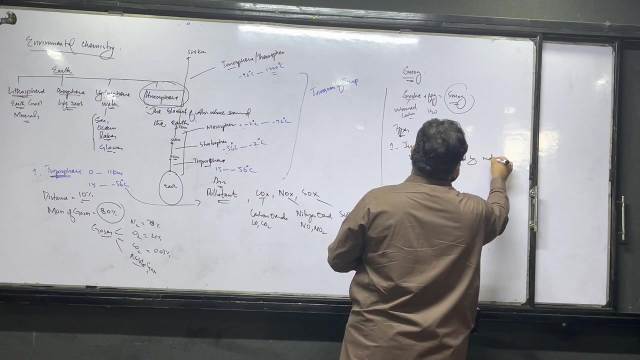 Now children, the smoke is different types. When we look at the smoke, they are different types. So the very first one is the industrial smoke, The smoke which is produced by due to the industrial waste. I say that the smoke is actually produced by the industrial waste. 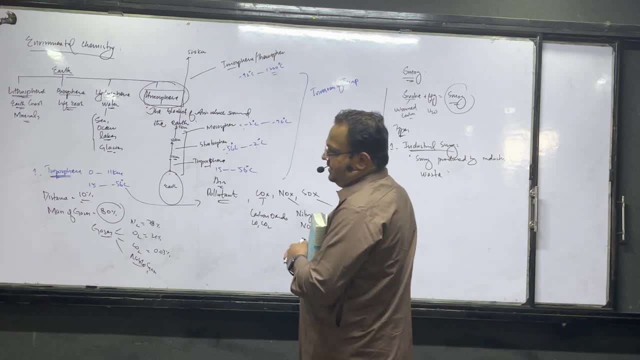 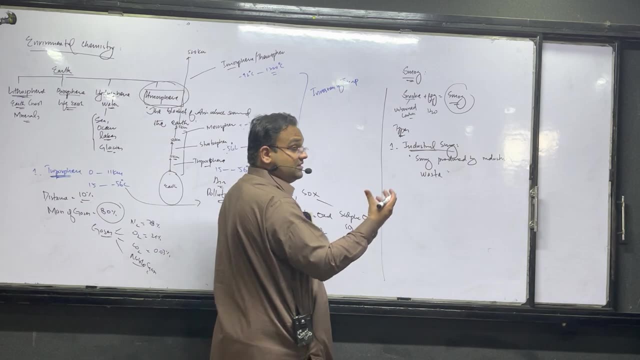 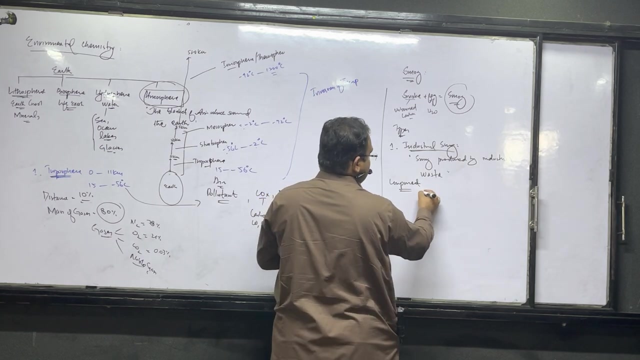 So that smoke is actually called as industrial smoke. Now in industrial smoke, what are the most important things, What are the problems, What are the components of the industrial smoke, What is its composition? So in industrial smoke, many things are there. 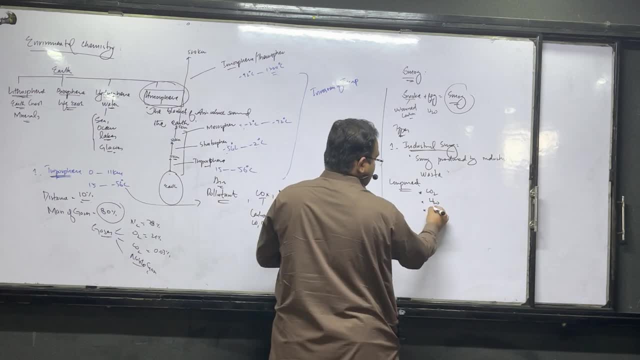 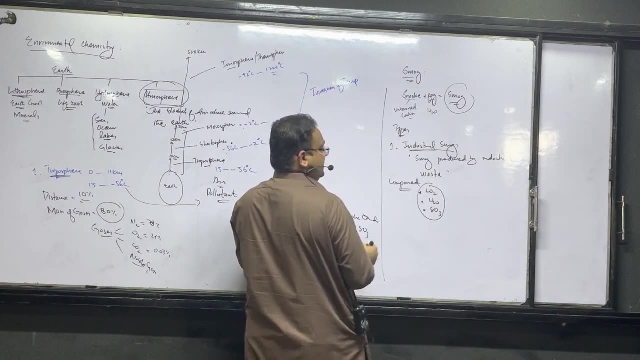 One is the unburned carbon dioxide, And what is the second one, Water, And the third one, Sulfur, Dried Outsides. These three together actually make what Industrial smoke, And the color of this is called. 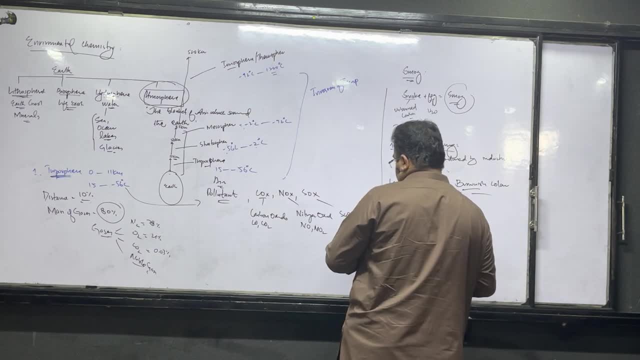 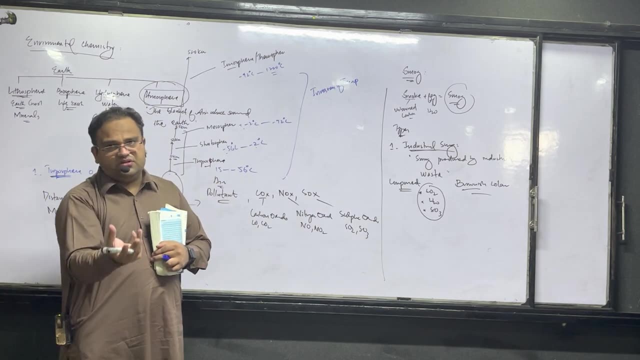 it is the brownish color. What color is it? Brownish Student, do you know that when there is smoke there are different types of problems? Okay, in this class there was a little bit of a problem. You cannot drink sulfur. 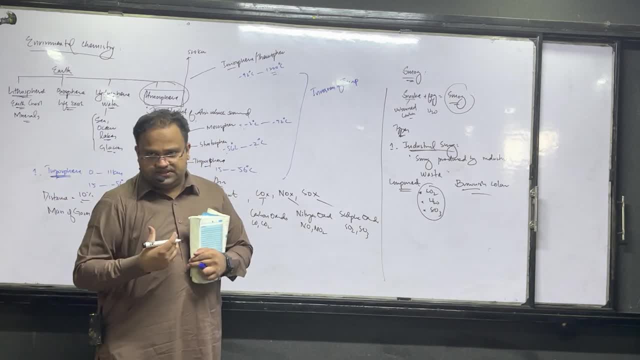 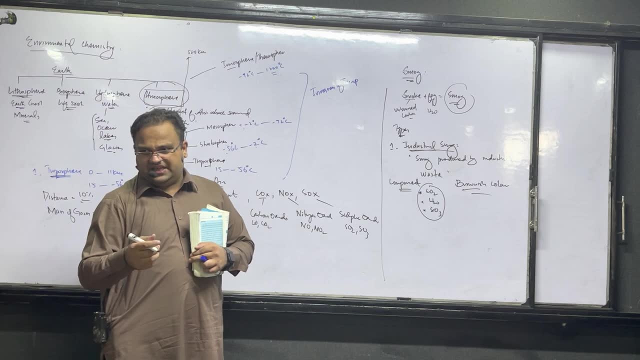 But apart from that, they can cause different types of lung diseases. Right, students, Lung diseases. we have different types of diseases. Yes, sir, Not to mention necrosis, etc. These kinds of diseases Which are caused by industrial smoke. In Australia and America once the duration of the smoke from 15 to 30 days. because of that, different kinds of deaths are caused: Those who have asthma or asthma. for them it is very dangerous Anyhow, 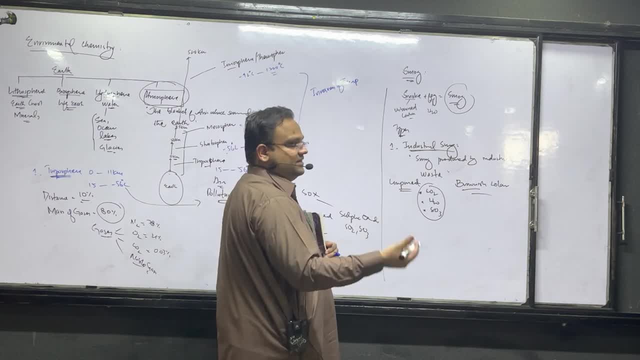 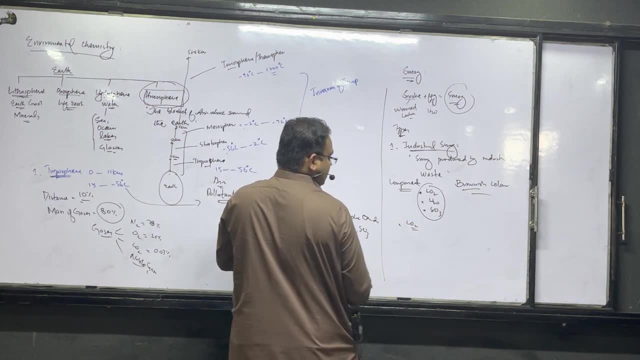 this smoke is really called as industrial smoke. Okay, this is called industrial smoke. It comes out of the smoke And in that smoke, actually, what is present? Carbon dioxide In the smoke. usually coal is used, Coal is set on fire. 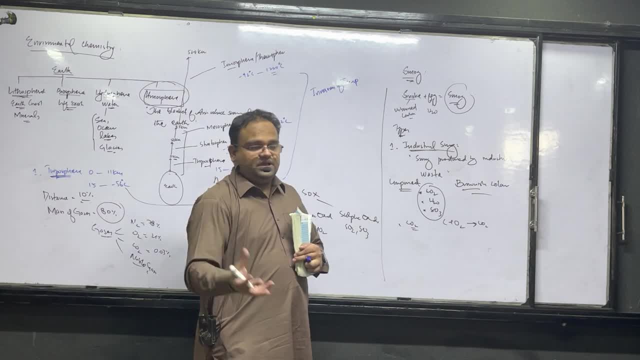 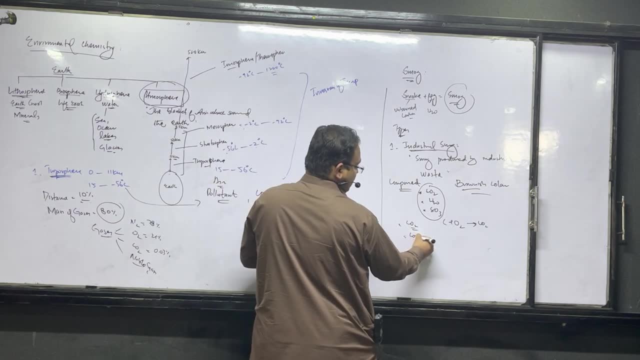 and how is it made? When it produces heat, it is used because, as a result, what is made? Carbon dioxide is made. And let me tell you one more thing: In coal, sulphur is also made. What is made in coal? Sulphur. When you burn coal, sulphur reacts with oxygen to produce sulphur dioxide And sulphur dioxide. many times it reacts with oxygen to produce sulphur dioxide. So, all these coal, the smoke that is created on us. 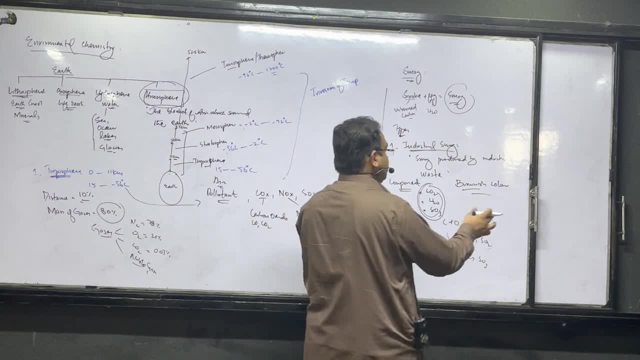 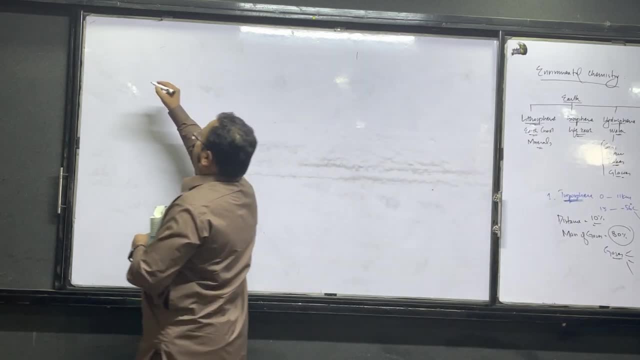 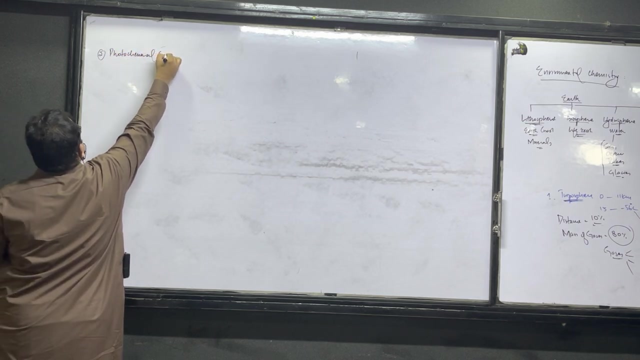 that is generally called industrial smoke, The other type of smoke, second type of smog, that is here The second type of smog, So that one is called as photochemical smog. This is a polluted process when it is polluted. it causes these types of pollution: Photochemical smog. Now let us say that the smog produced due to light Point of view, the smog produced due to the light, So that smog is called as: 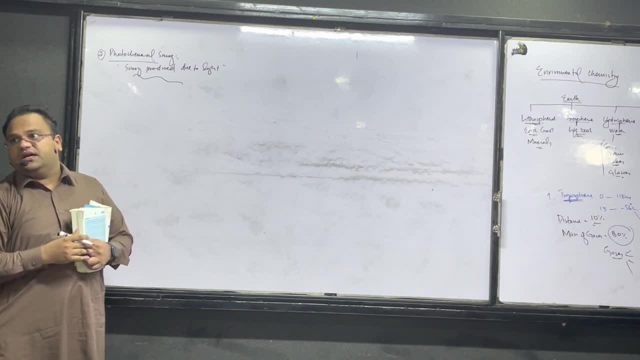 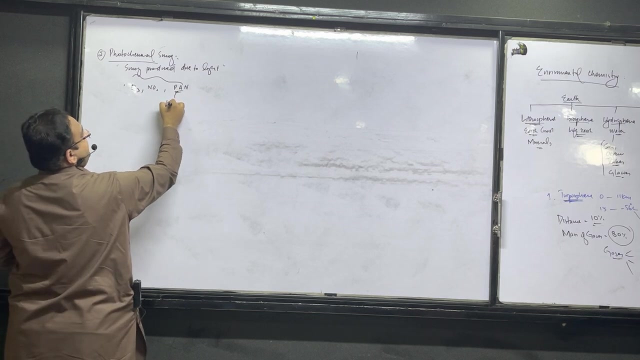 photochemical smog. It is called as photochemical smog. What are its major components? Its major component is ozone, Apart from that nitrogen dioxide. And the third thing is PAM, And PAM corresponds as a. 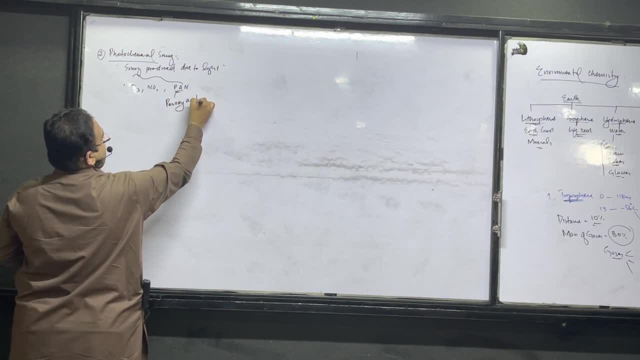 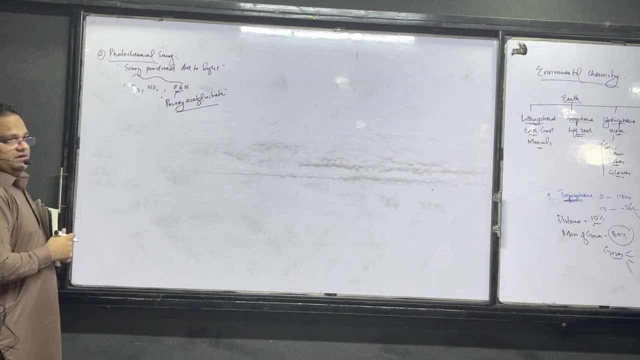 peroxy n-c-ti- nitrate. What is written in all the books? PAM peroxy n-c-ti- nitrate. These three together create the smog that is called as photochemical smog. 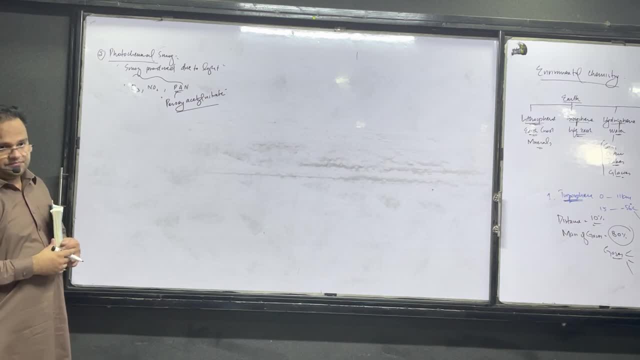 But how is it produced? Children will get it In the air. nitrogen dioxide is produced. So in the presence of light, nitrogen dioxide is decomposed into nitrogen monoxide and oxygen. So in step number two, oxygen is made of. 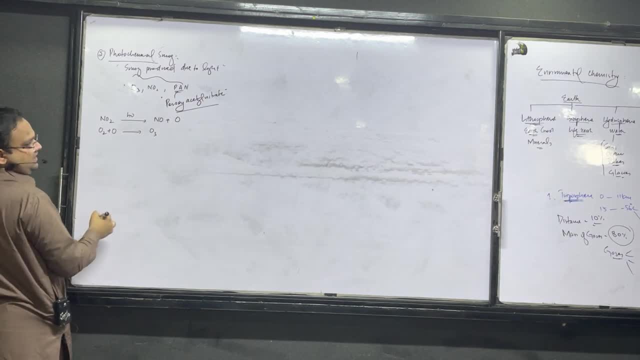 oxygen, and oxygen is made of oxygen. So tell me what is actually being made here? Ozone In the air. there are alkanes, Alkanes, RH, Which you also call as hydrocarbon. What do you call it? 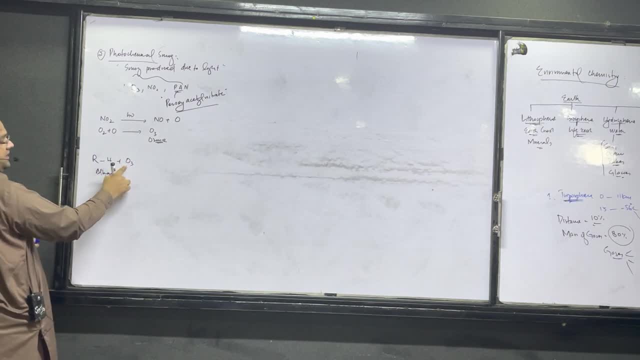 Hydrocarbon. So this ozone, this ozone, by reacting with this alkane, you will have carbo-oxidant radical. What do you call it? Carbo-oxidant radical, Carbo-oxidant radical? Look at here. 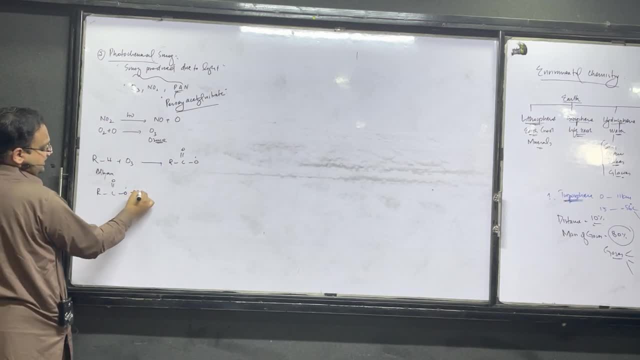 This carbo-oxidant radical, again by reacting with oxygen. we have R-C-R-O and O. Now we have per-oxy-acetyl. What has been made? Per-oxy-acetyl radical In the next step? 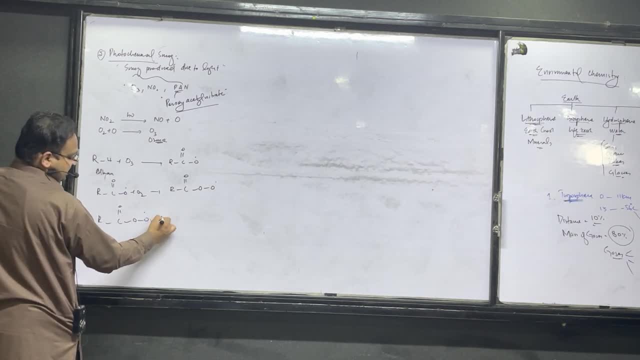 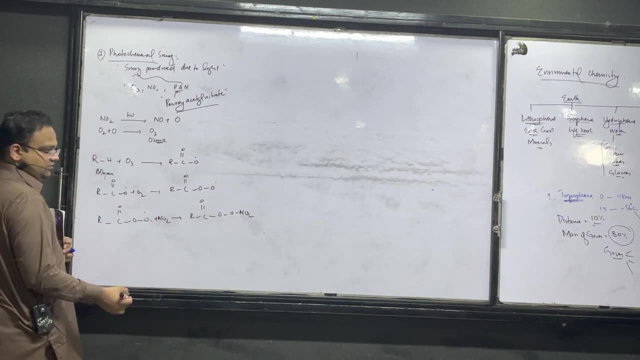 with this per-oxy-acetyl, radical nitrogen dioxide will react and you will have this R-C-R-O, and here we have nitrogen radical NO2.. And this alcohol is actually called as PEN. What is it called? 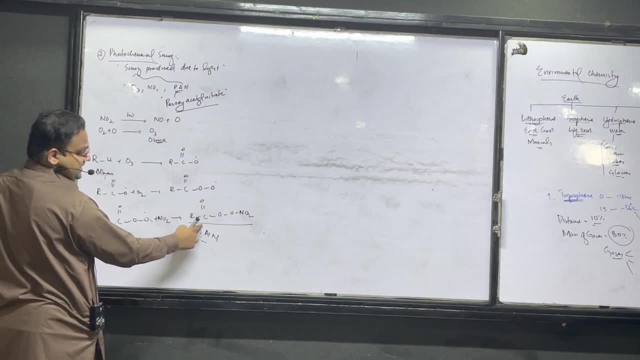 PEN. Now, what does PEN stand for? R-O-C-E-C-E-T-I-L-E-N-I-D-R-E-T. All of you say R-O-C-E-C-E-T-I-L-E-N-I-D-R-E-T. Everyone clear. 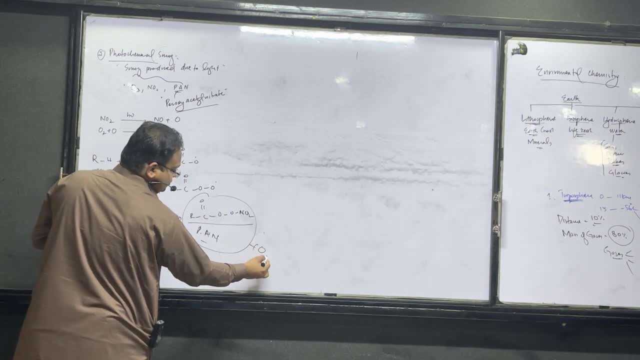 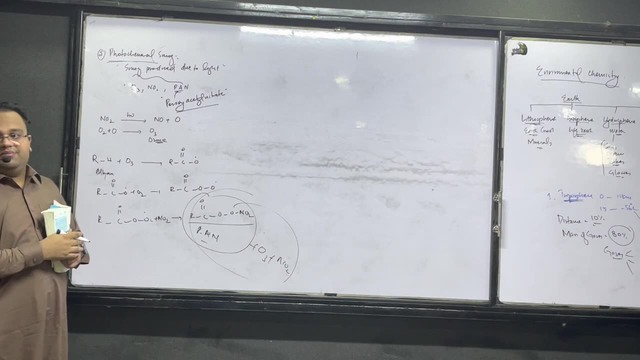 Now this thing, this PEN, plus ozone or plus nitrogen dioxide, all of these, what can be used to generate this one? Can we move on to the next one? R-R-R-R-R-R-R-R-R-R-R-R-R-E-T-I-L-E-T-I-N-I-N-I-N-I-D-R-E-T-I-N-I-N-I-T-I-N-I-N-I-T-I-N-I-T-I-N-I-T. 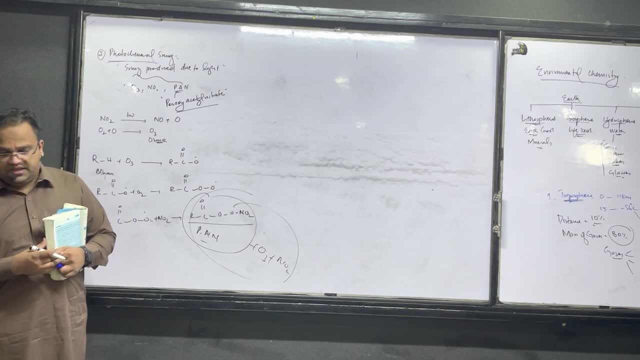 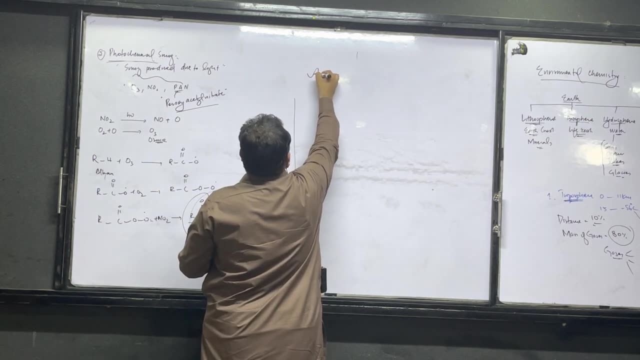 And this is a kind of air pollution. This is a kind of the air pollution. This is a kind of the air pollution. This is a kind of the air pollution. Okay, Now listen, There is another topic, and that one is the. 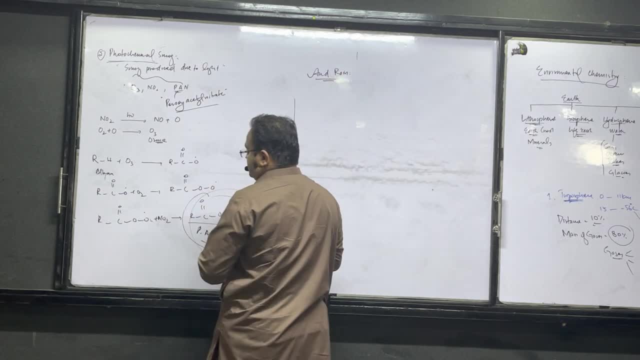 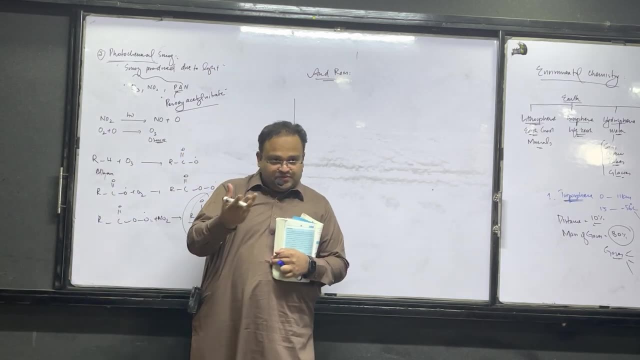 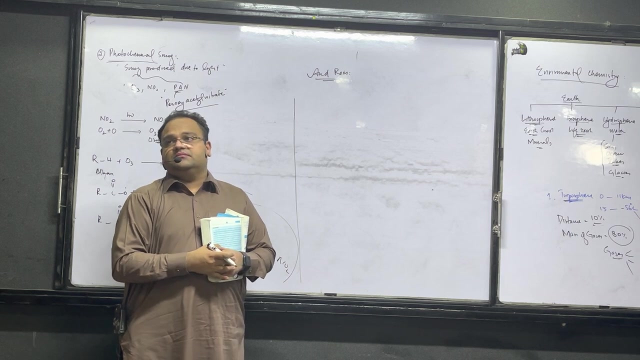 acid rain. Okay, When it rains water, water comes out, Water comes out. Do you know the answer? When it rains a lot. When it rains a lot, See, there is a little acidity in the rain, Of course, 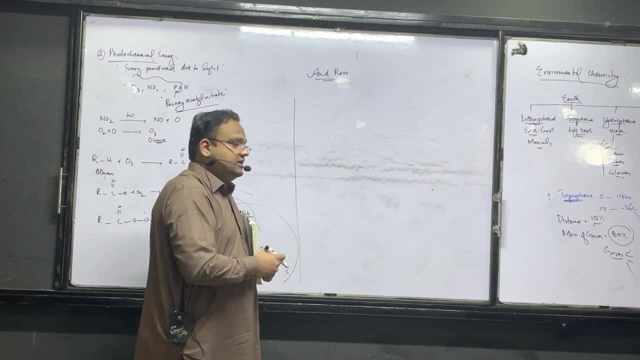 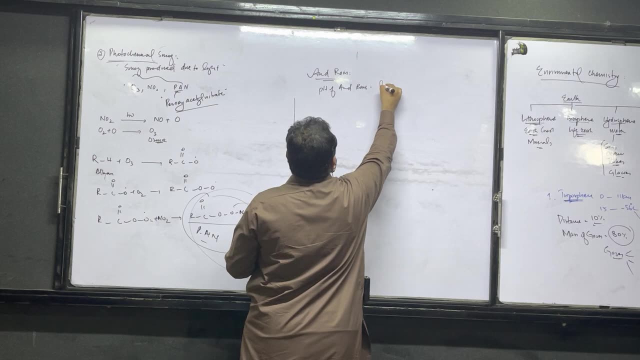 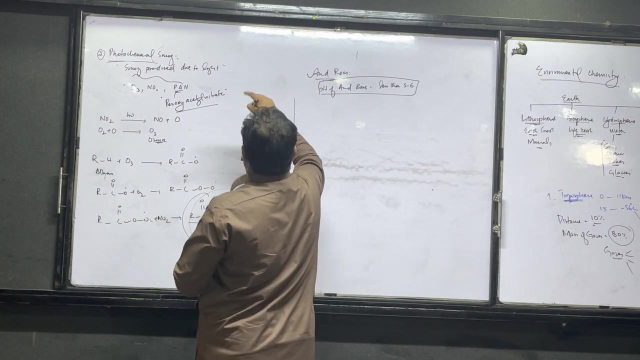 what is actually called acidity in the rain. The question is: what is the pH of? What is the pH of acid rain? The answer is less than 5.6.. What is the answer? Less than 5.6.. And if you ask me, what is the pH of normal rain? What is the pH of normal rain? What is the pH of normal rain? 5.6 to 6.. The answer is: keep in mind, the pH of normal rain is 5.666.. 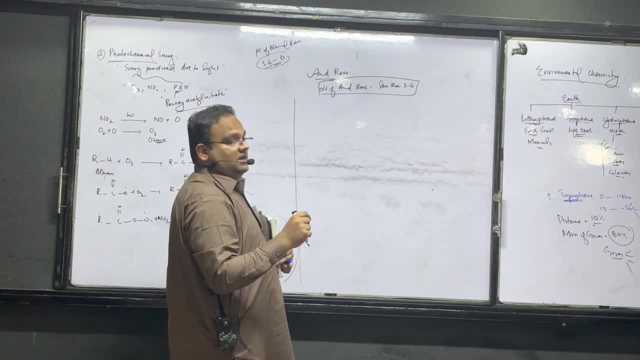 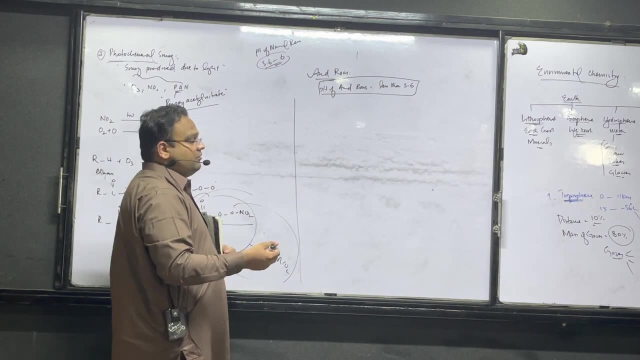 And the pH of acid rain is less than 5.6.. Now, where does the acid come from in the rain? Now, where does the acid come from in the rain? I told you that there are pollutants in the air. Now, what are the pollutants? 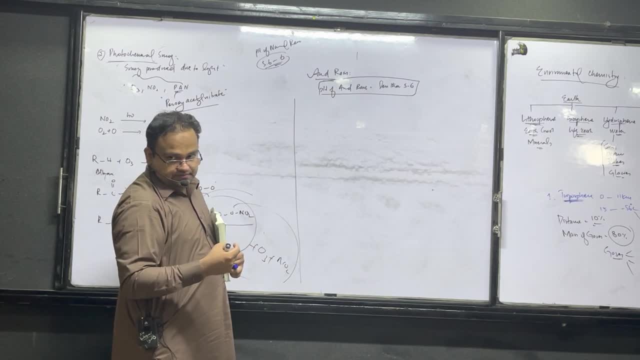 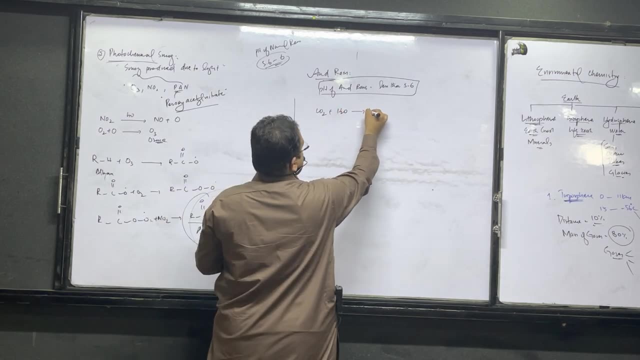 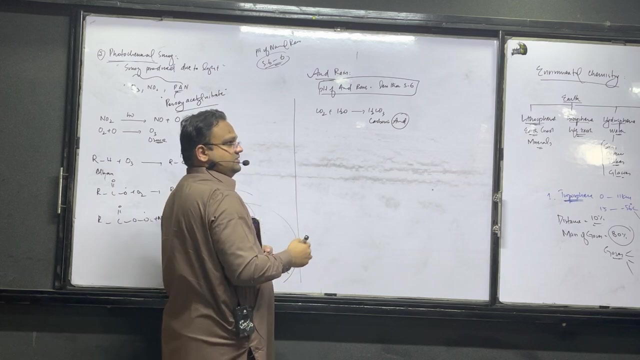 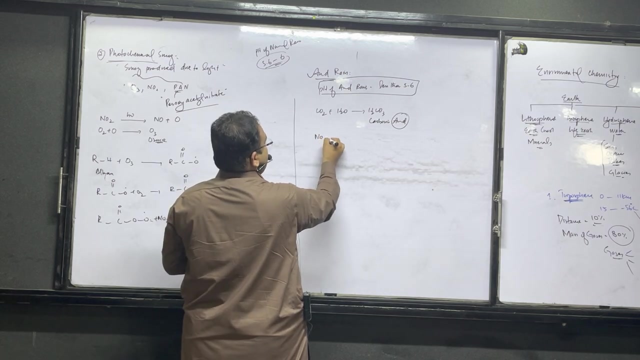 COX, NOX, SOX. So this carbon dioxide reacts with water and makes carbonic acid. And what is this carbonic acid? This carbonic acid reacts with water and makes COX, NOX, SOX, SOX, SOX, SOX, SOX. 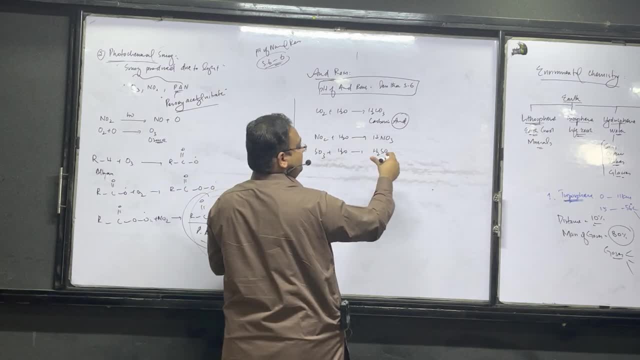 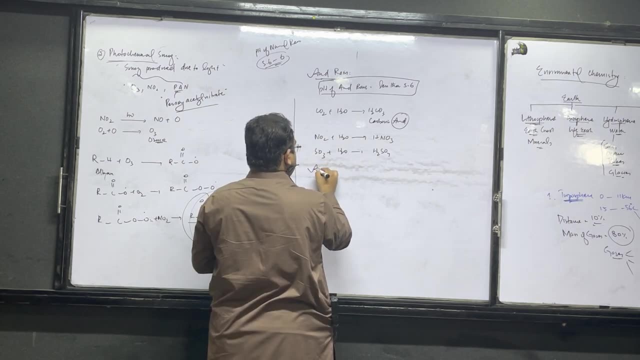 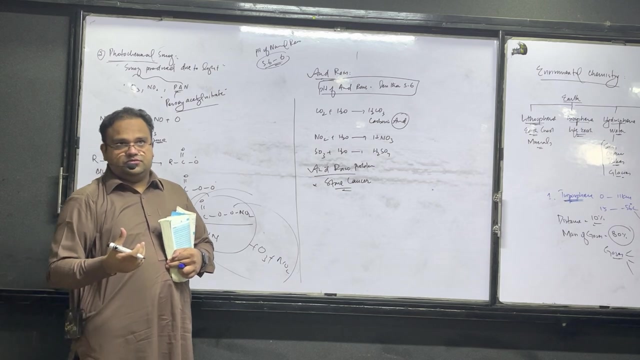 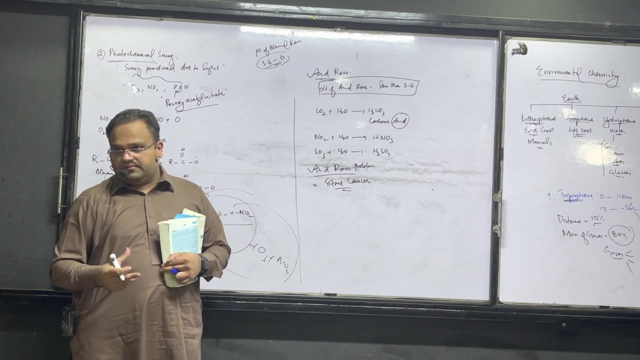 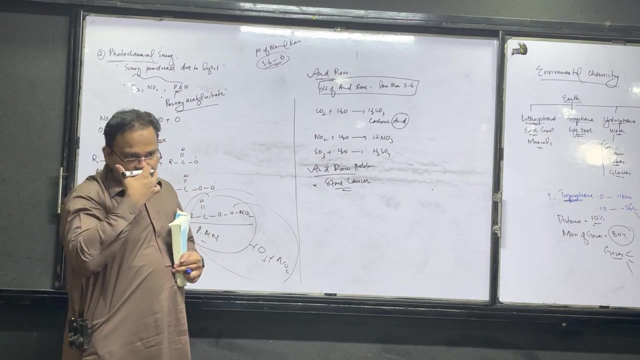 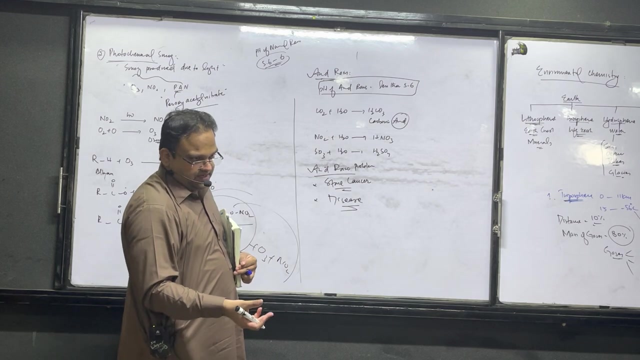 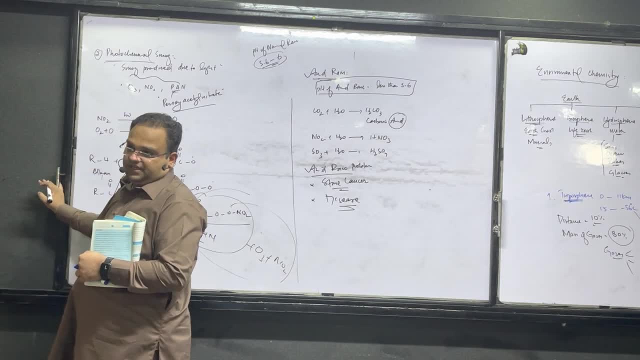 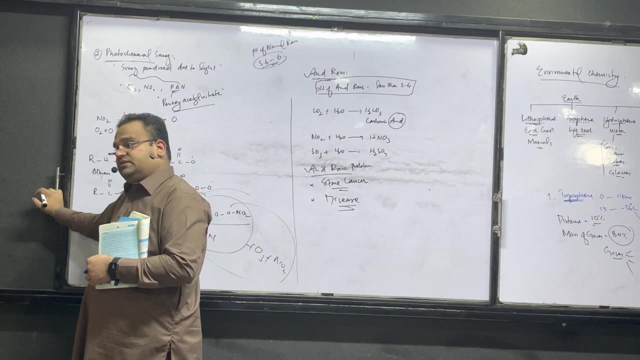 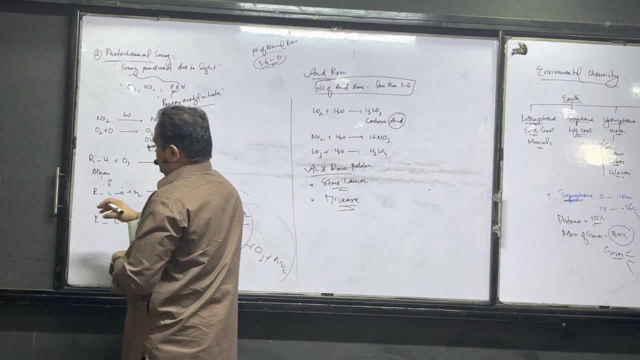 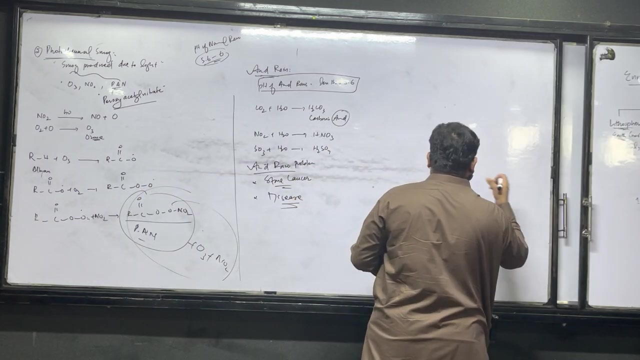 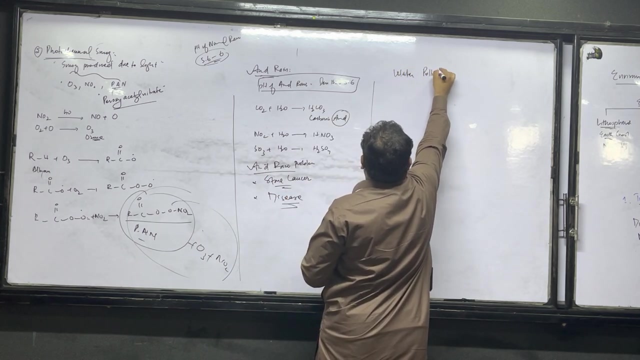 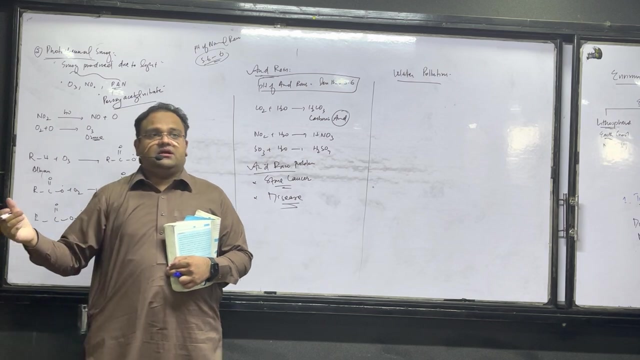 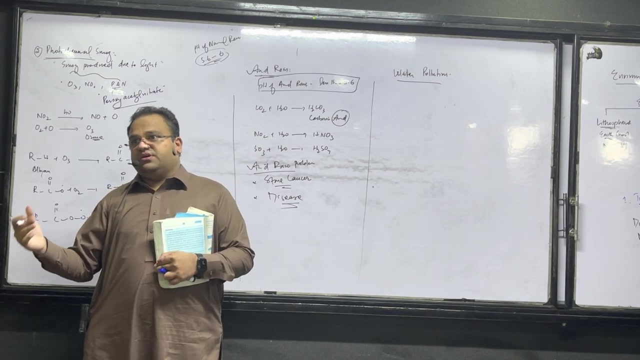 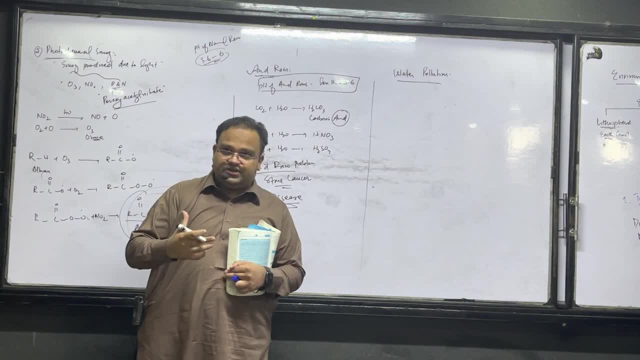 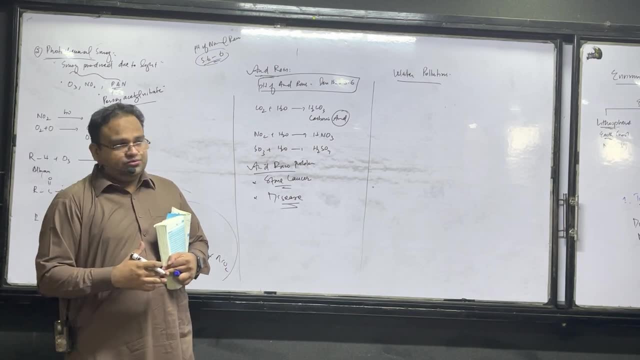 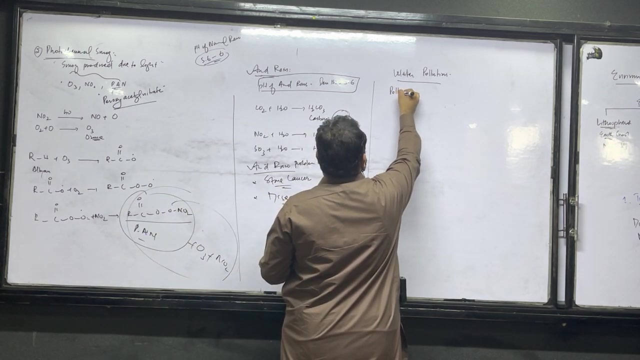 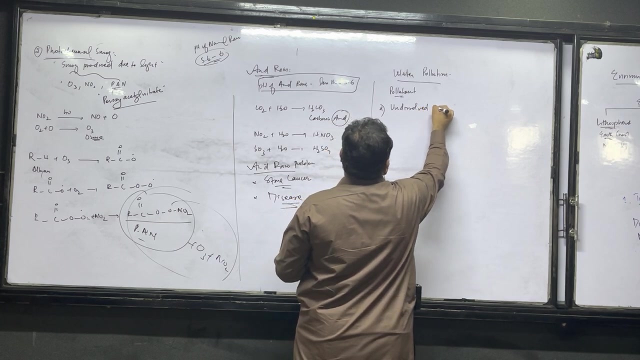 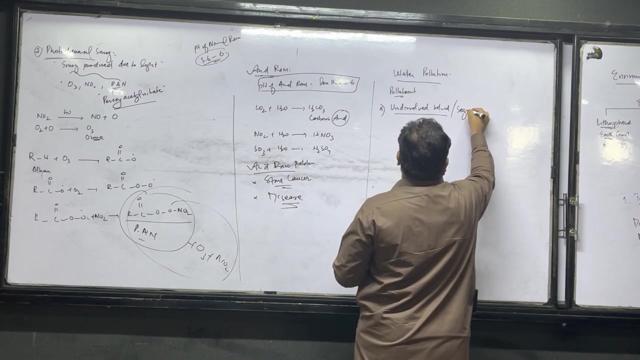 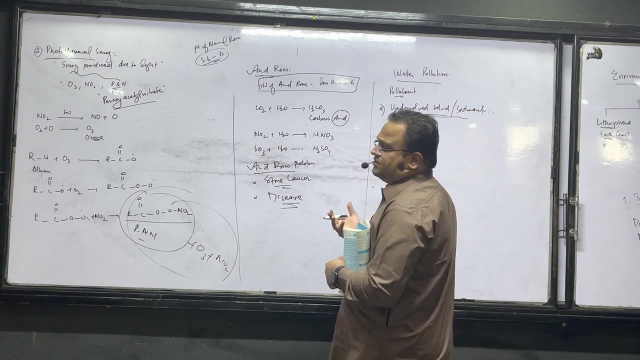 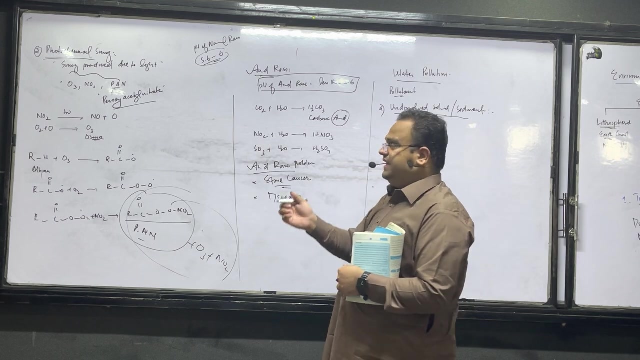 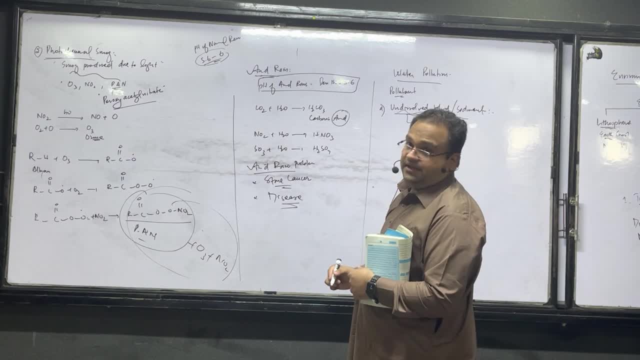 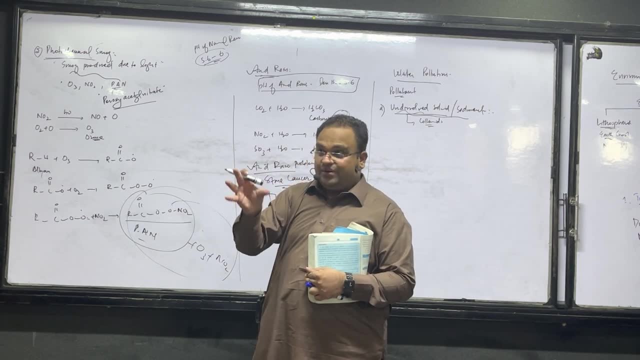 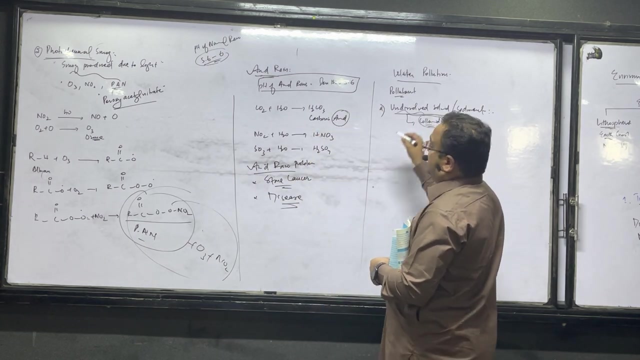 SOX, SOX. You have never seen a canal before. Obviously you don't see anything like that, but it is not clear, it is not transcribed, So the thing that is present in the Mujibutti is actually a variety. 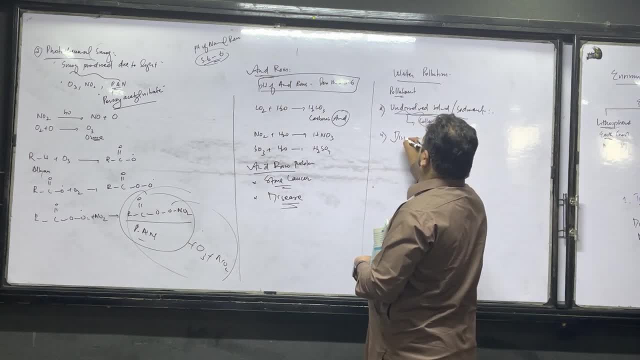 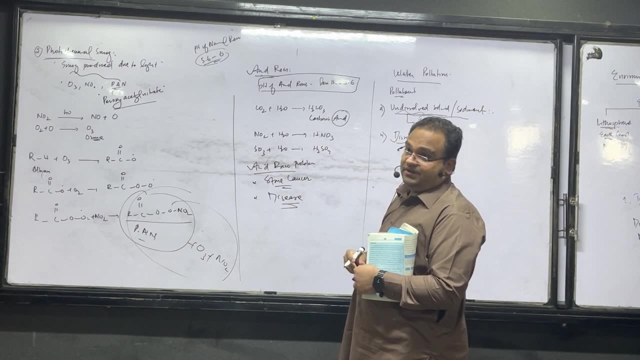 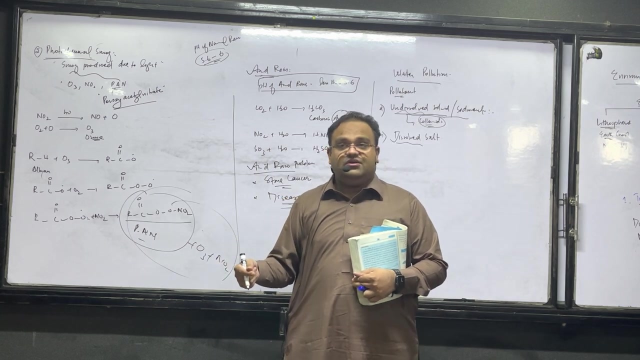 The other thing that is present in it is Resolve Salt. What is the name of that? Resolve Salt? It is a little bit like a poster. You have to take a bath in a poster. So tell me, while taking a bath in a poster. 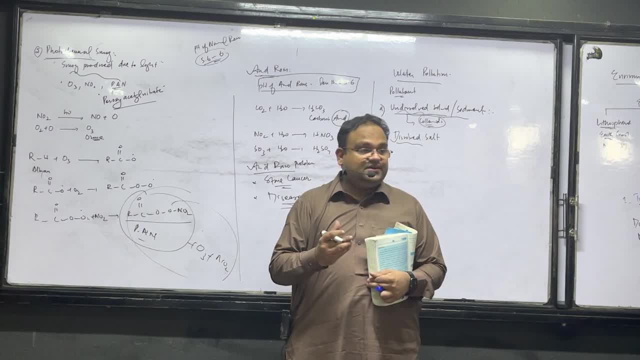 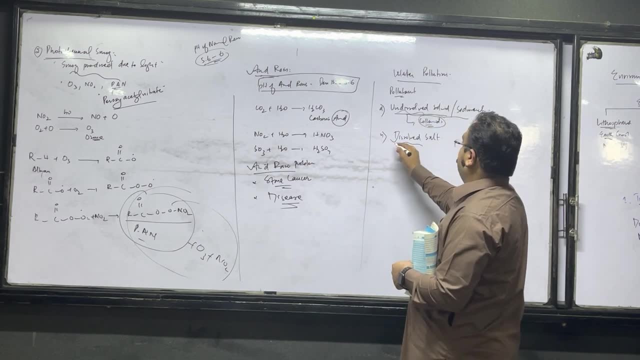 there are white, white particles below. These are the dissolved carbonates. What is dissolved Dissolved carbonates? So the second thing that can be polluted in water is: what is dissolved salt? What do you have in it? There are carbonates. 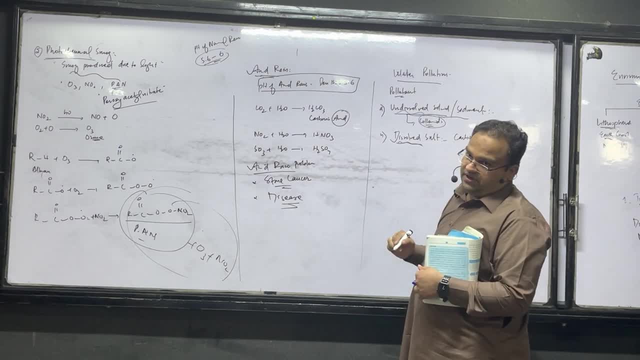 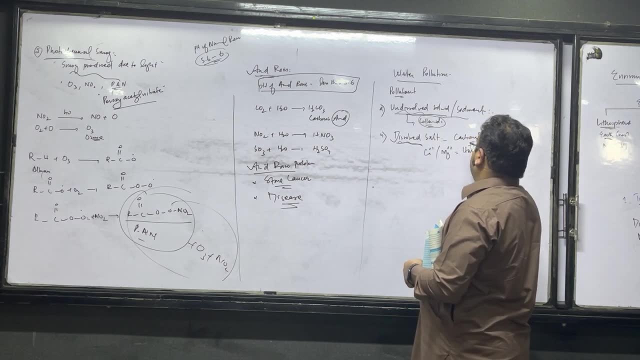 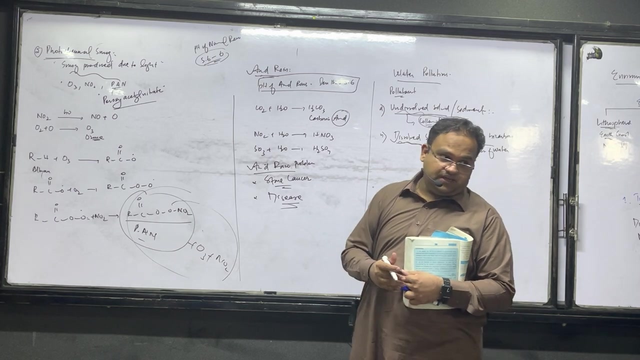 You have carbonates outside And so on, And so it is. And, apart from that, if it contains calcium ion and magnesium ion, then remember, it causes the hardness of the water. It causes the hardness of the water, So all your expenses will be increased. 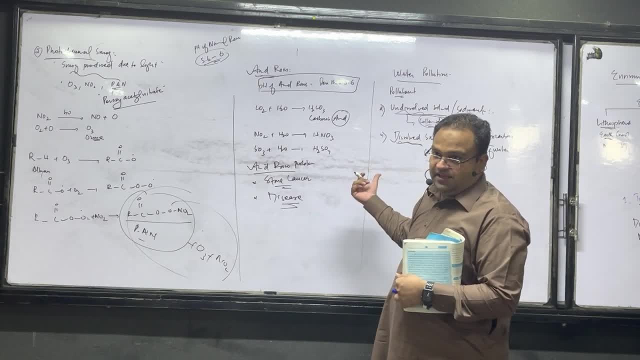 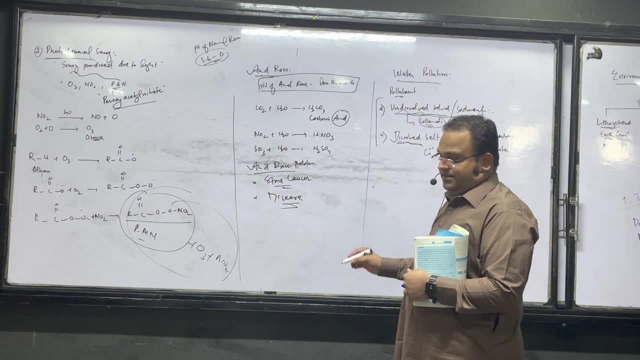 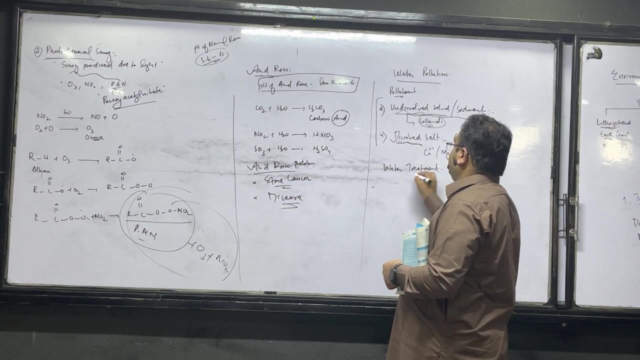 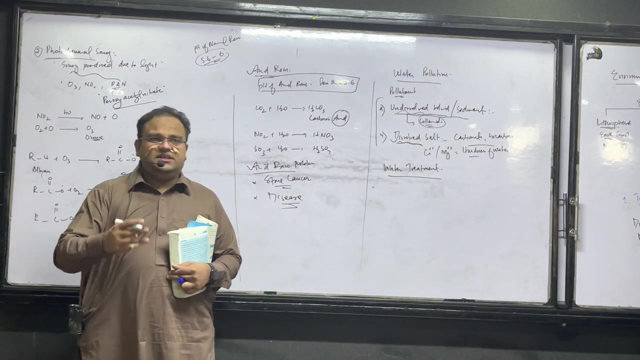 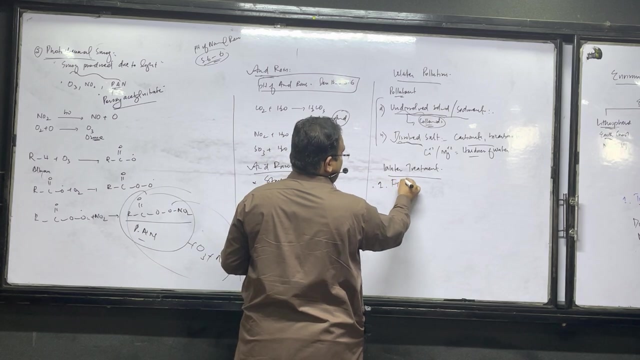 Now to remove these things. water is treated with it, And that one is called as water treatment. Water treatment means to clean the water. How do you clean the water? There are three steps. The first step is: what will you do with the water? 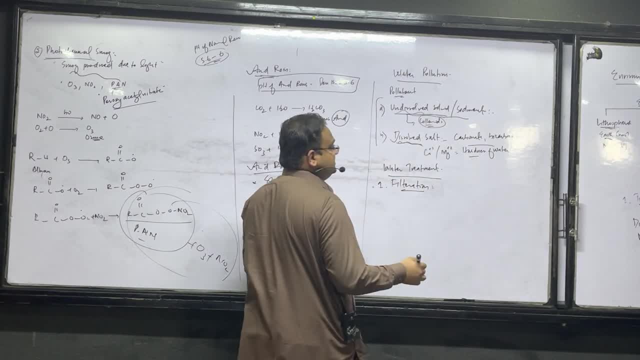 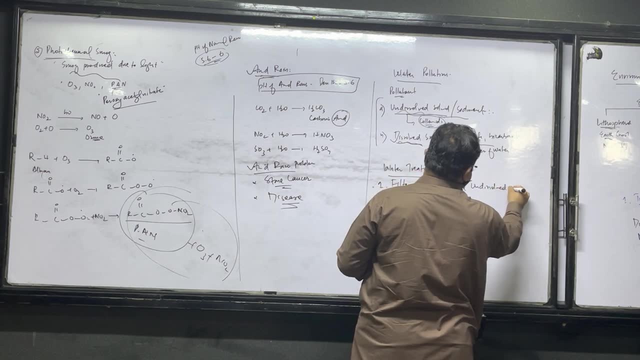 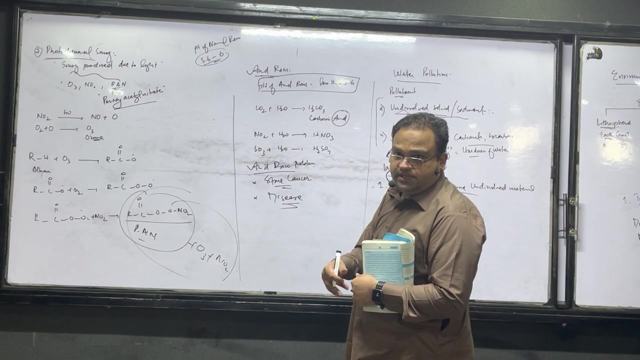 Filtration. What will you remove from the filtration? You will remove the undissolved material. What will you remove from the filtration? The undissolved material, The sand will be removed. But even now there are some products available. 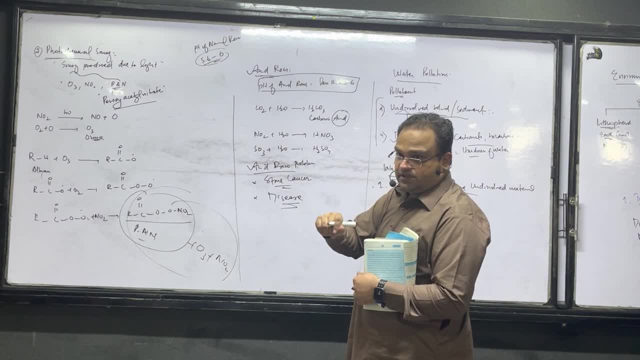 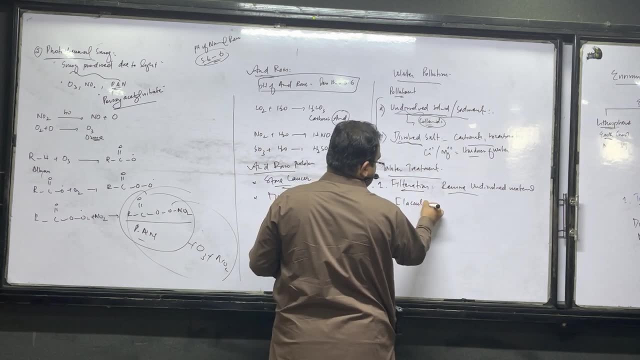 If you don't want to filter it, you can filter it with a filter wiper. The second thing you will do is flood ventilation. What will you do? Fluctuation, Fluctuation, Fluctuation. This is called poavulation. 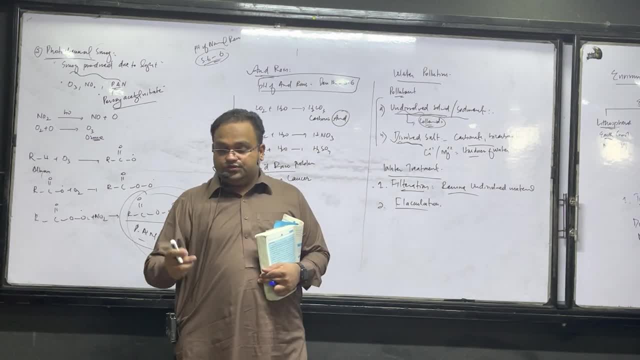 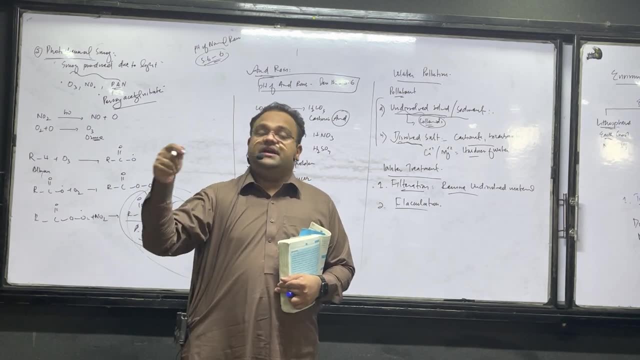 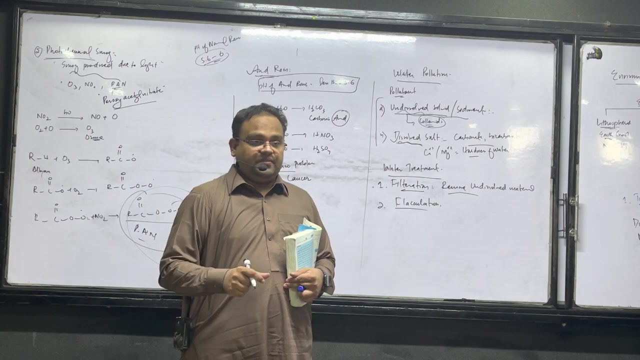 What is poavulation Student in the water? the water is poured with pitcubic acid. Pit-a-tray, Pit-a-tray. What will that do? It will remove the opaqueness, the collides. It will remove it. 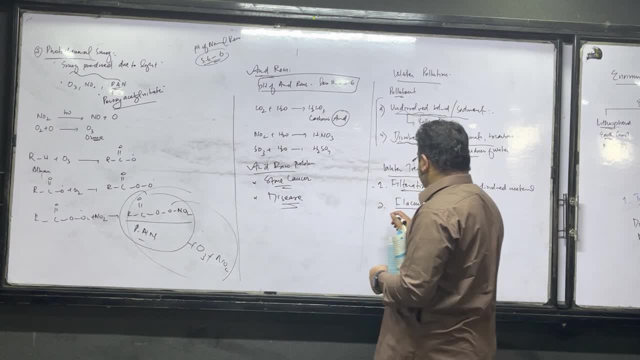 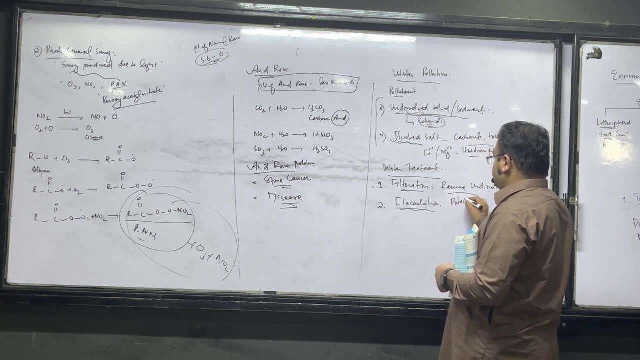 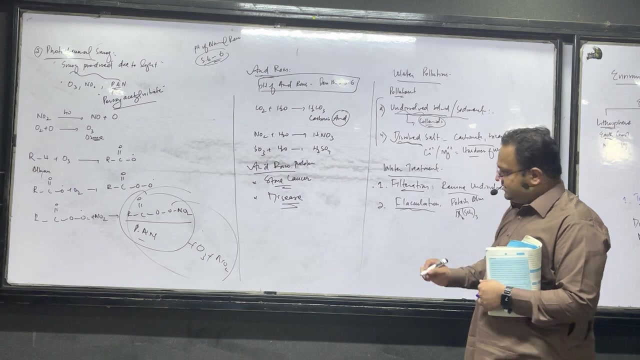 What is this process called? It is called Potassium. What is it called Potassium? The major component in it is the Aluminium Sulfate. What is Potassium Sulfate? It is a double side. It is a double side. 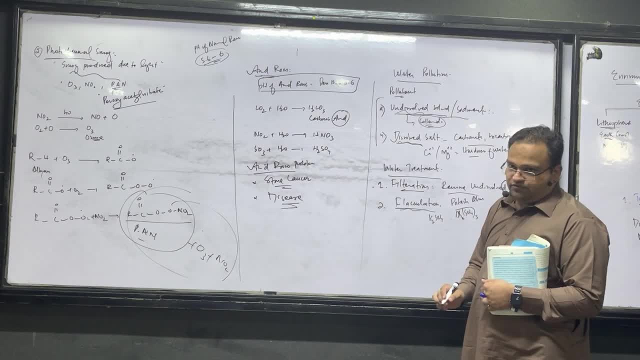 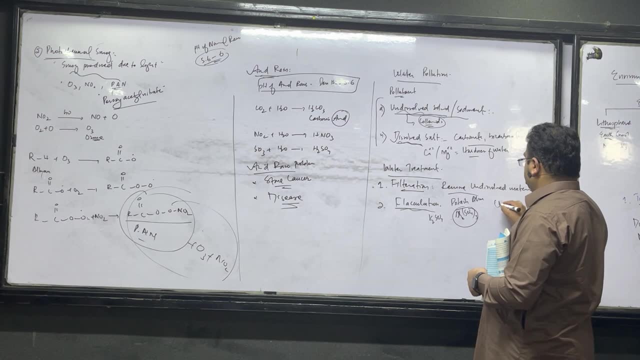 Potassium Sulfate is called K2SO4 and Al2SO4. But what is the major component? Al2SO4.. And do you know, The opacness or the cloudiness of the water is basically calcium hydroxide. 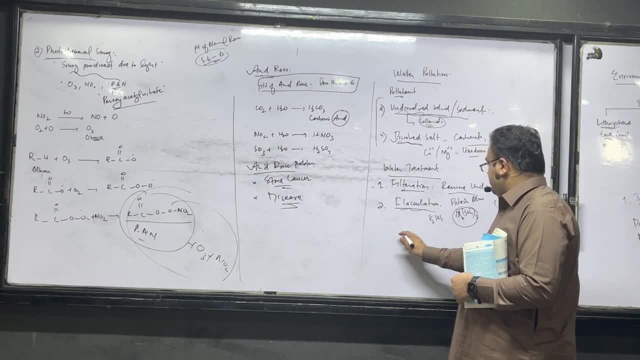 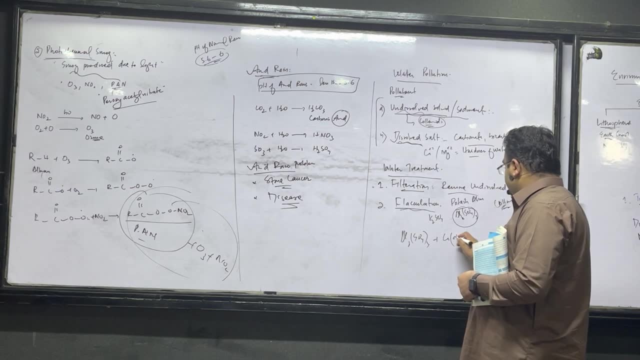 What is calcium hydroxide? Calcium hydroxide: When you put potassium carbon in it- ie Al2SO4O3, it will react with this chloride, And when you put potassium carbon in it, it will turn it into Al2SO4. 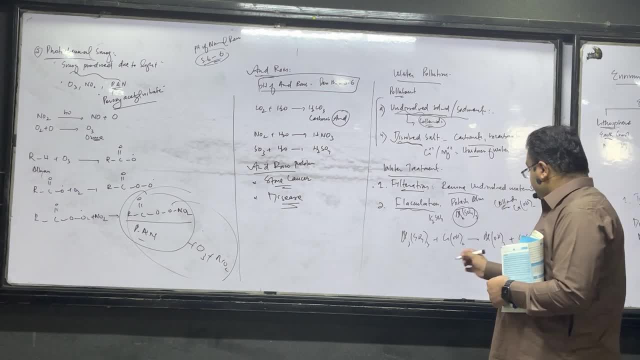 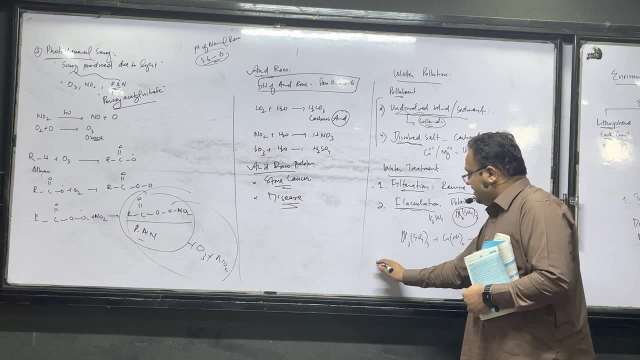 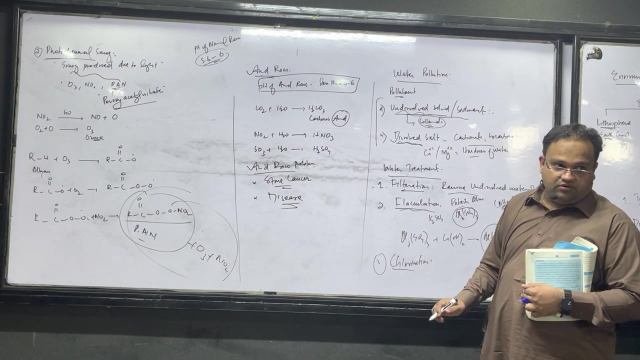 And it will turn it into calcium sulfate And this Al2SO4 will be removed in the form of precipitate Right student. And the third treatment you will do is Chlorination. What will you do? Chlorination? What will you do? Remove bacteria. 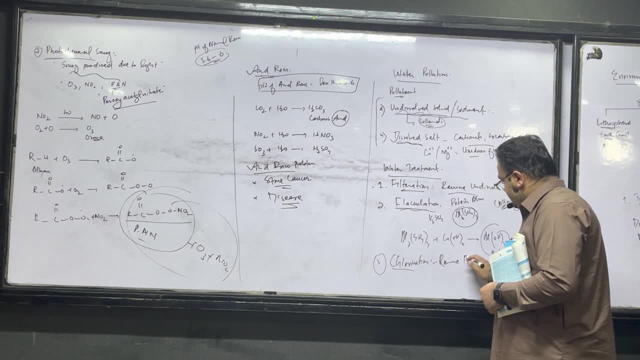 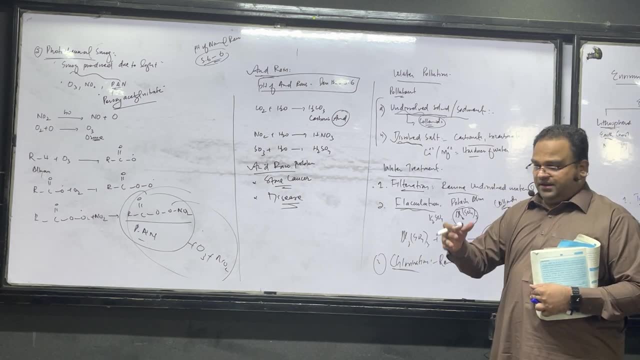 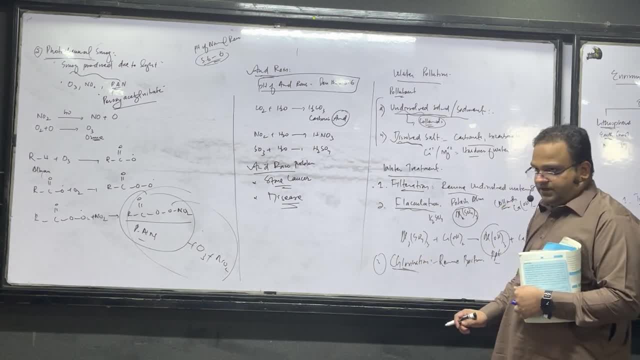 you told me that, your friend, when you put water in a container, you put water in the container, it will hydrate it. What will you do? It will actually turn chlorine. What will you do? One important thing is when you put chlorine in water. 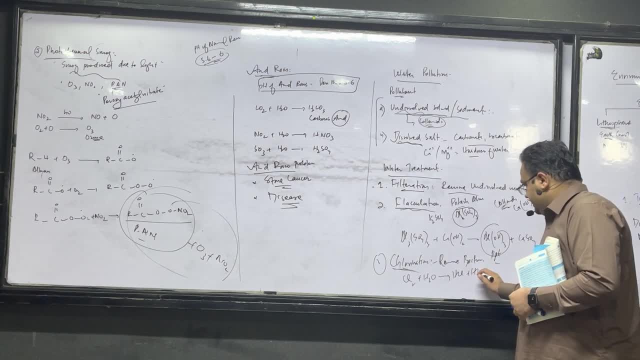 we have learned this in organic chemistry. Tell me what it makes. HCl plus HCl- we have learned this. And HCl it decomposes into a light structure. N to HCl plus oxygen. Can you write it? It is a house. 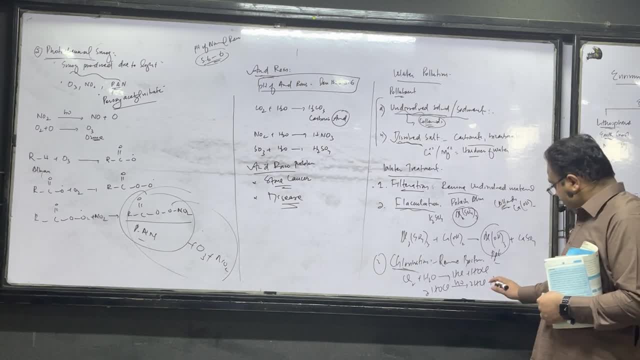 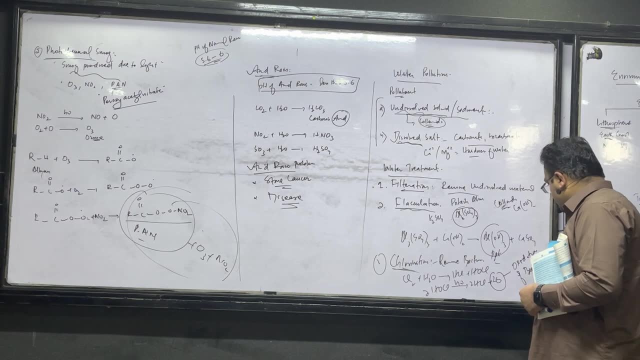 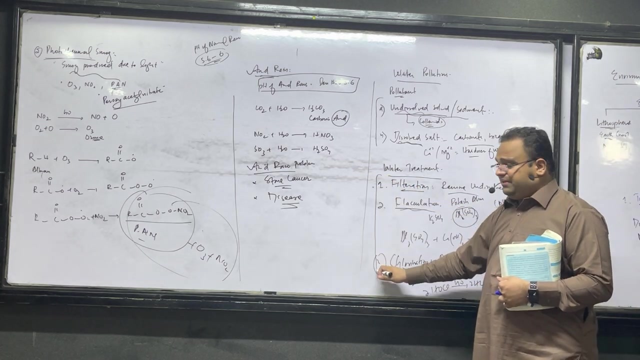 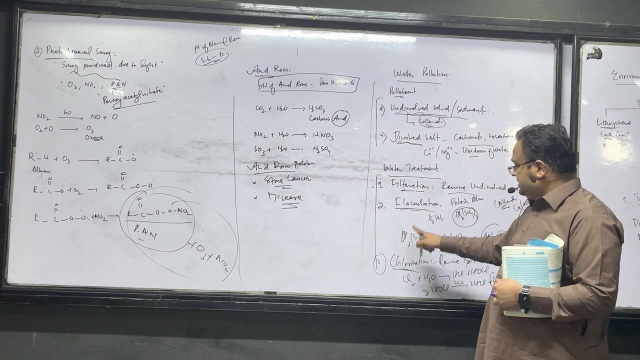 after into the air, In that This oxygen is used for the oxidation of bacteria and they will kill the bacteria. The water treatment is session one, To remove the colitis And third is to kill the bacteria. So what happens to the water? 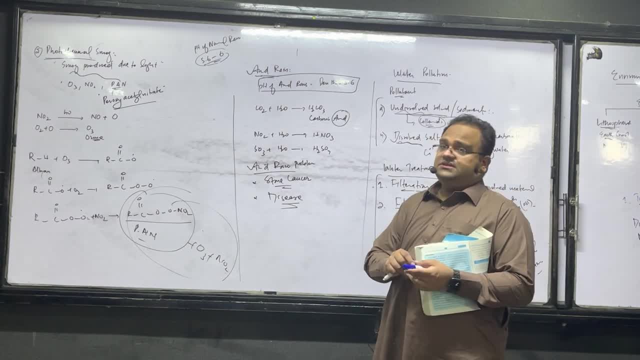 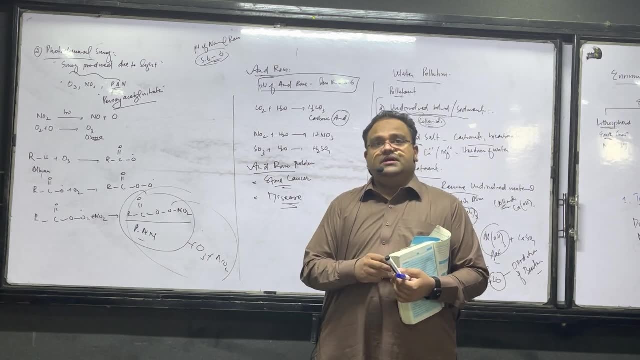 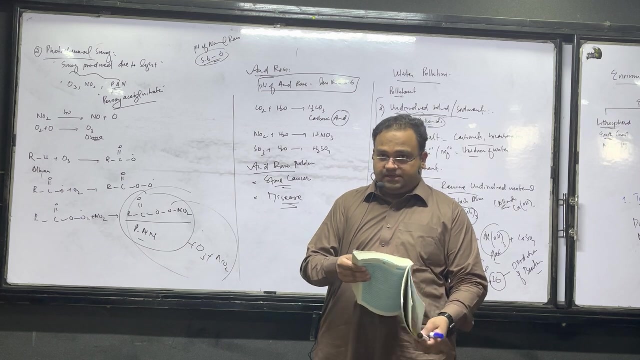 We want to clear. These are the topics which were included in the environmental chemistry We want to clear. So these were the topics And We will say that you have done a very good job And marks are good And your interest is good. 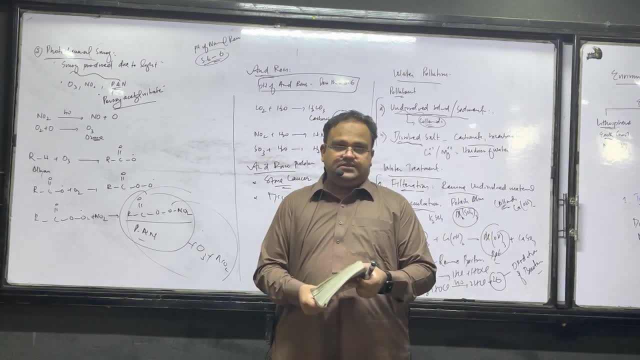 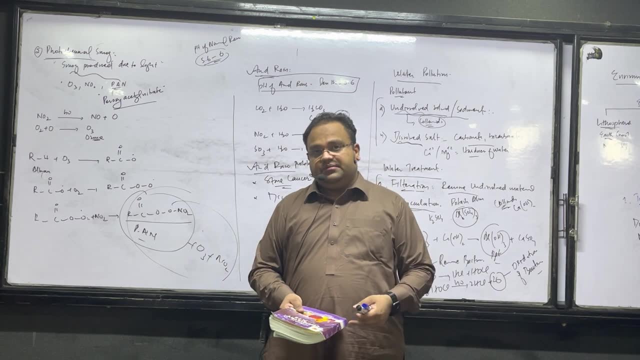 And this is an admin- And from July the classes will start. If you want to attend the classes, The admission is starting from now. You can do admission. It will be a 45 day situation. We will start the admission course according to the BMC syllabus. 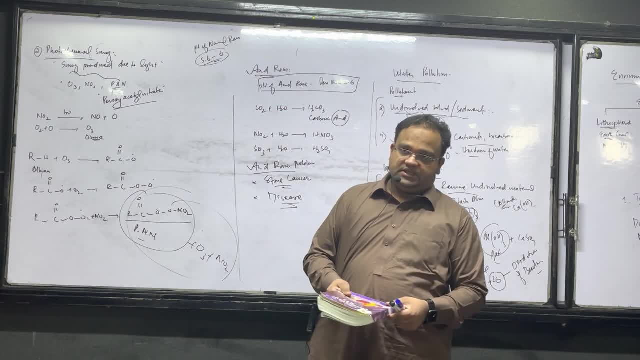 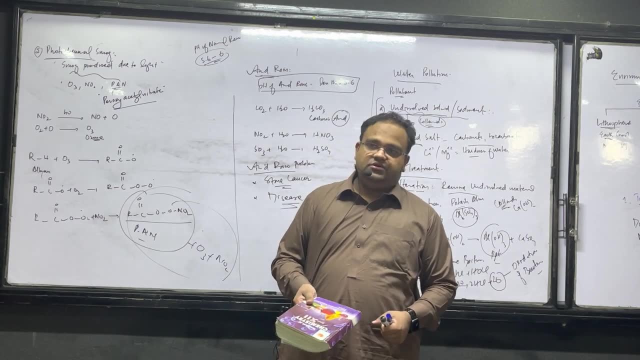 Okay, Thank you sir. So if you want to take admission, So you can take admission from now, So that you can move forward with the first classes, Our investment group will take your position. Thank you very much. Thank you, sir. Thank you sir.